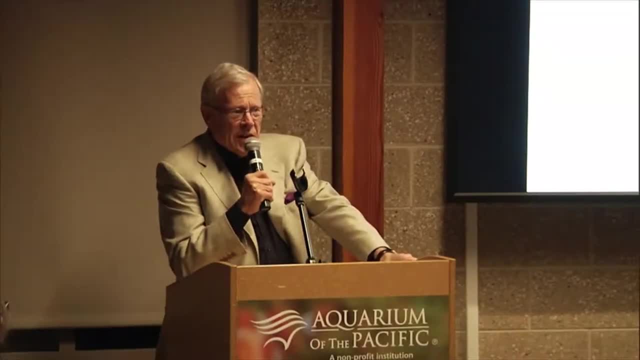 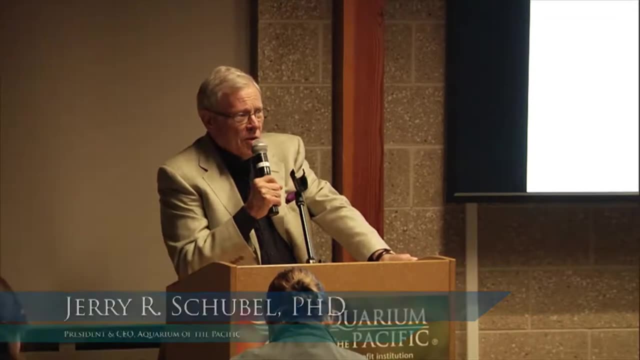 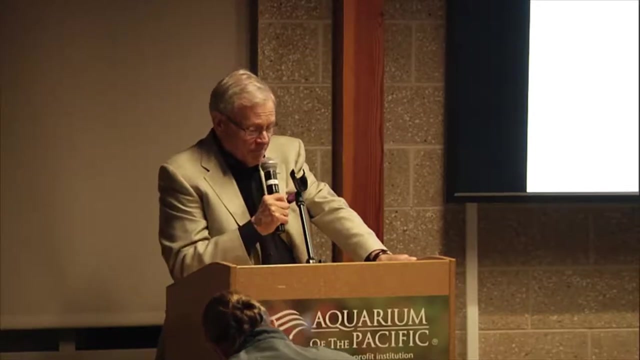 So tonight we're going to hear about ocean acidification and then we're going to hear about coral reefs and the major threats to coral reefs, one of which is ocean acidification. Our two speakers are both professors from Scripps, and Dr Todd Martz is going to go. 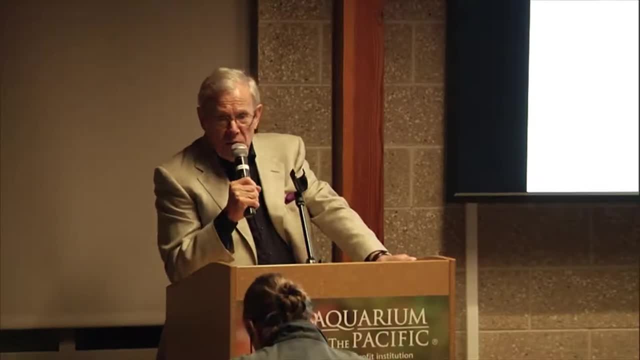 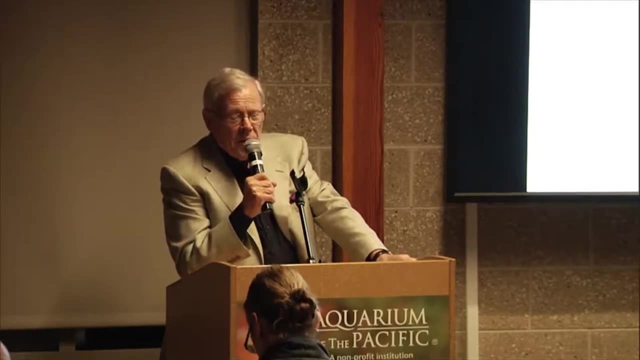 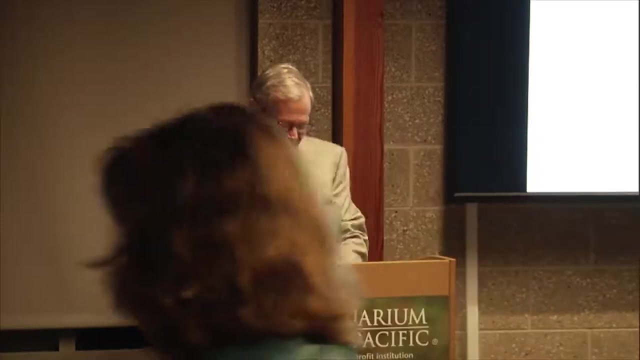 first, and you have their bios in your packets, so I'm not going to go through all of these, but just let me make a couple of comments. Todd and they've both been at Scripps now- for what did you say? Ten years, Ten years, Nine years, Nine years? Okay, And they went. 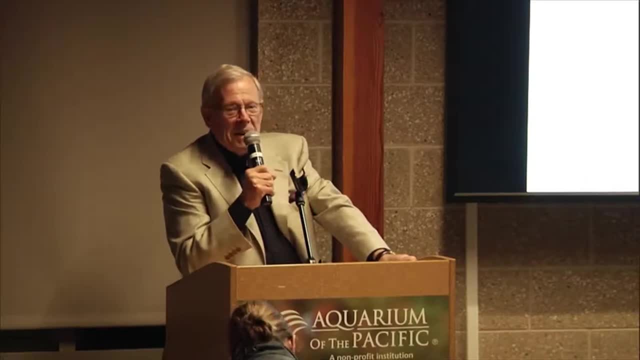 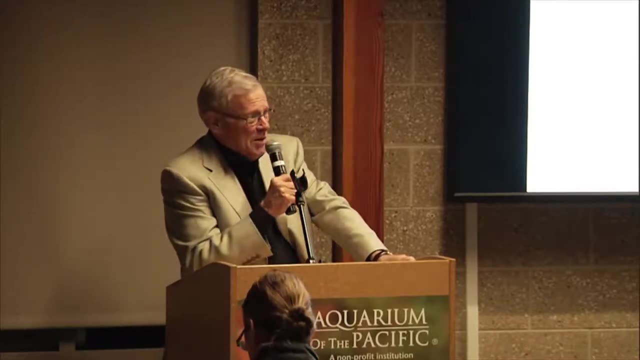 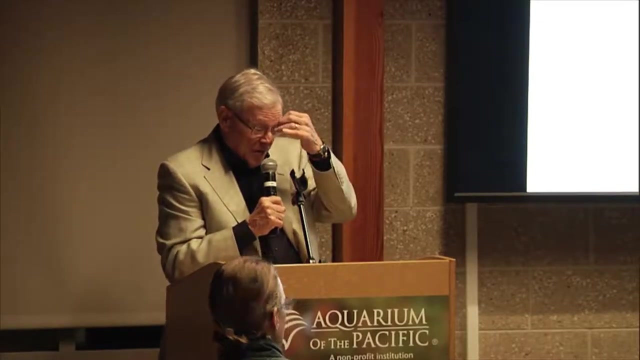 at the same time and Todd had been at MBARI that all of us know well, the Monterey Bay Aquarium Research Institute, and he was one of the beneficiaries of the OceanX Prize on pH measuring devices. And Jennifer Smith, her lab, studies coral reefs all over the world and looks at the 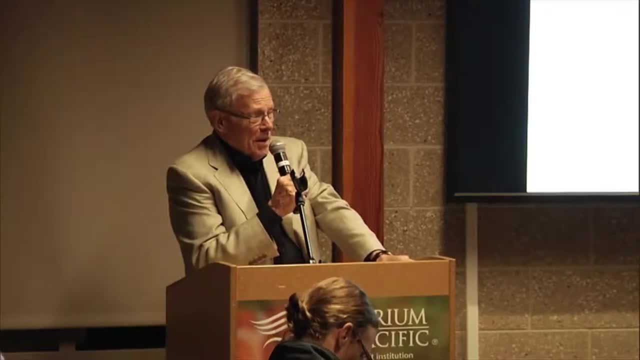 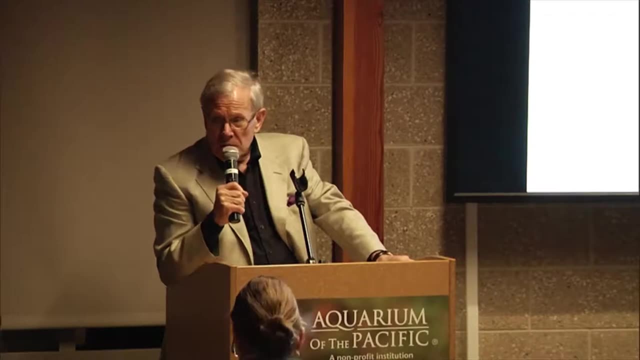 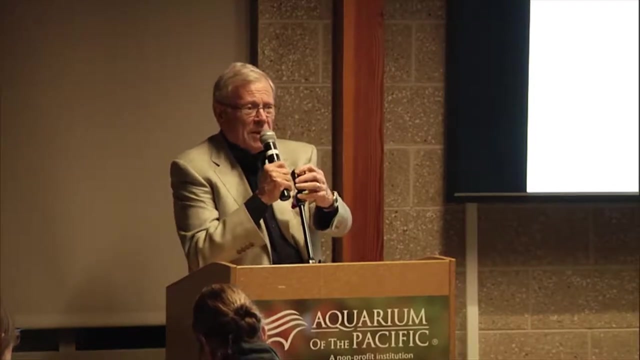 different threats to them, ranging from warming of the ocean, ocean acidification, but also things like fishing and coastal development and pollution. So Todd is going to go first, then we'll take a break and Jennifer will tell us about the world's coral reefs. So 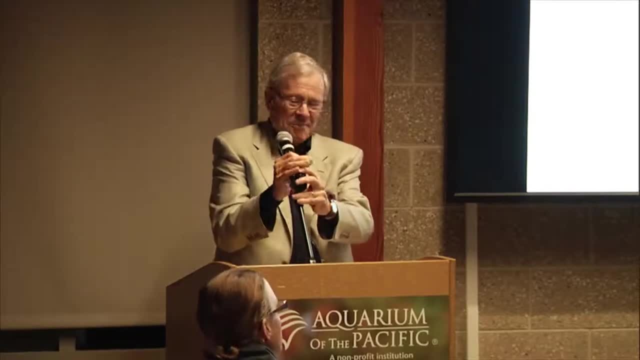 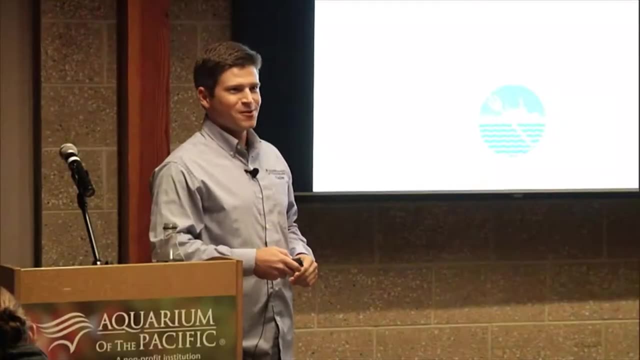 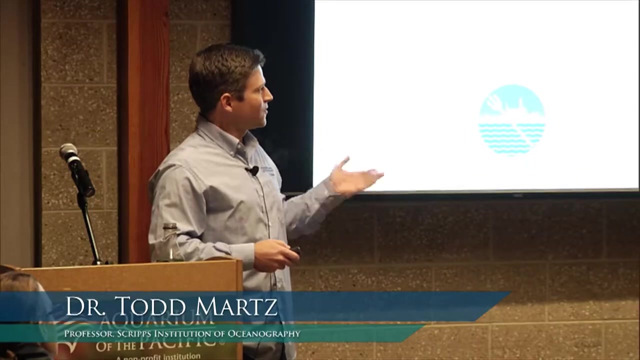 please welcome Todd Martz. Thanks, Jerry, first of all for the invite. We had a nice time walking around checking out the aquarium- really beautiful. I'm a chemist by training and I'm going to talk to you a little bit about marine chemistry just to start off, and I've kind of thrown 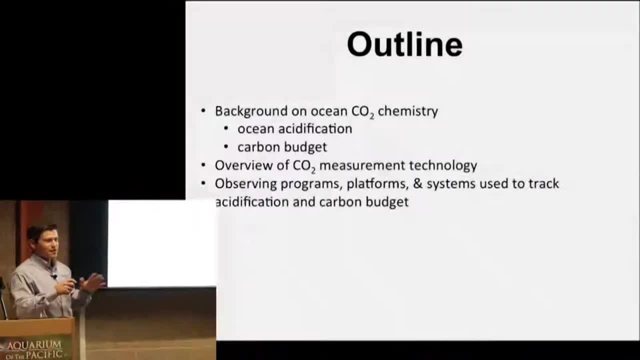 in three different topics here, which I hope they have some overlap, but I hope it's not too all over the place- But chemistry, background and talking about ocean acidification, which really falls under the larger umbrella of the carbon budget. So I'm going to talk to. 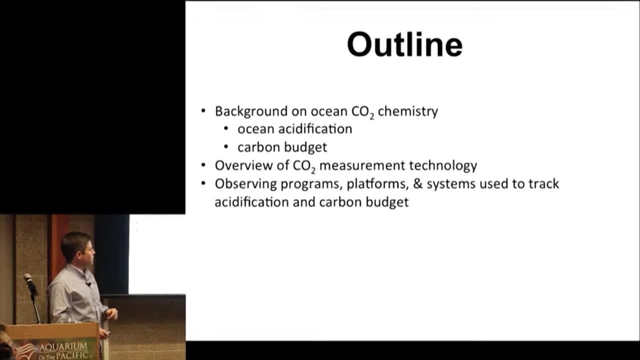 you about the carbon budget a little bit today, and then an overview of the CO2 measurement technology, which is really where I work. I focus on a lot of the engineering and developing new technology- sensor technologies- and then I'll try to pull it together with a discussion. 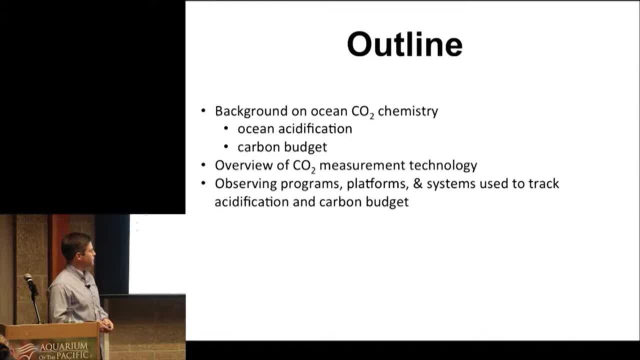 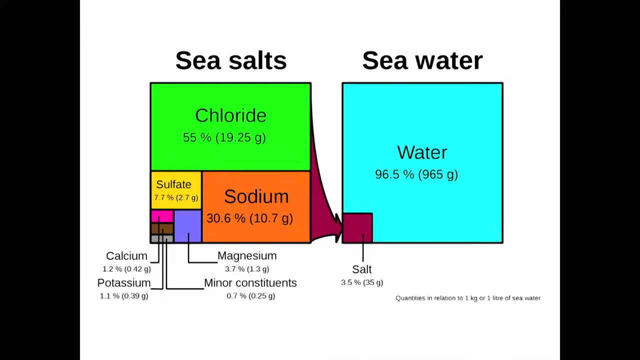 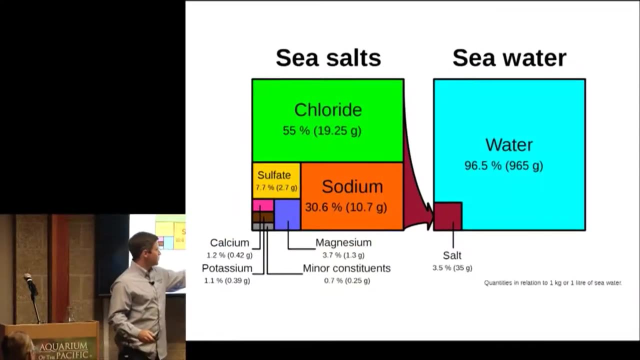 about some observing programs, past, present and future. So So if you haven't thought about marine chemistry in recent years, this is just a refresher slide to get us thinking about what's in the seawater And when we talk about salinity. 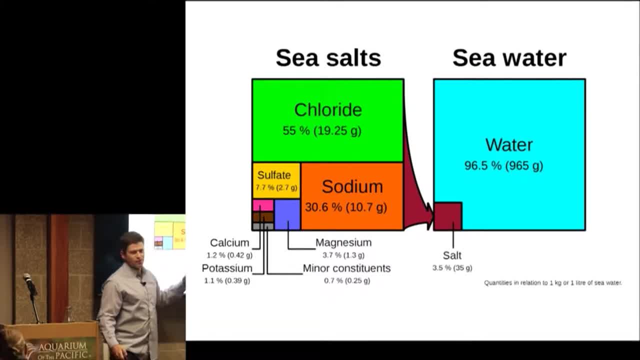 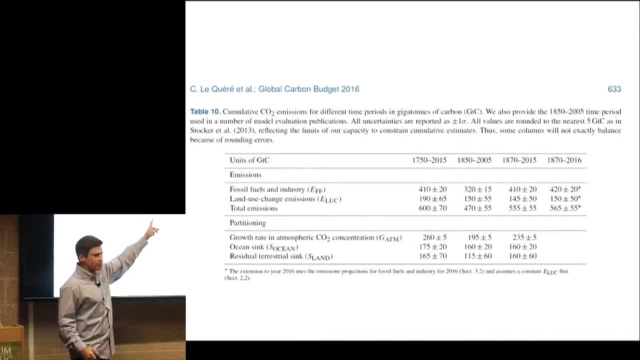 sea salt. And there's this little point in the ocean that's called the sea salt, And there's this little point in the ocean that's called the sea salt, And there's this little in terms of gigatons of carbon, about 600 or so. 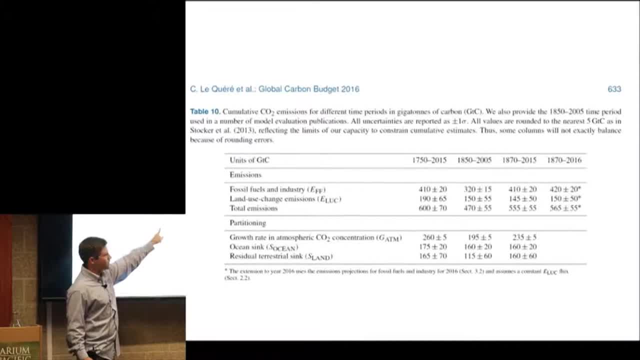 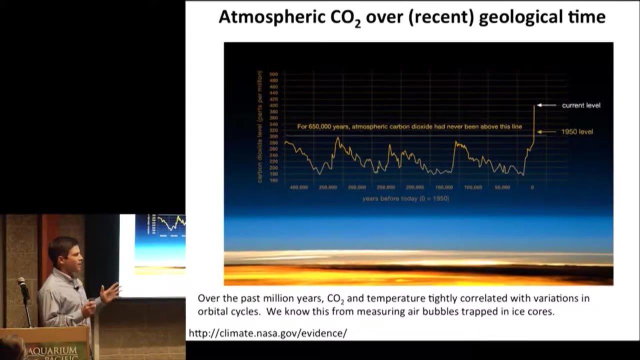 is the total amount that we've put in, we think, since the beginning of the Industrial Revolution, And most of that's happened in the last 140, 150 years. So that 600 number puts this into context. When we think a little bit about why scientists 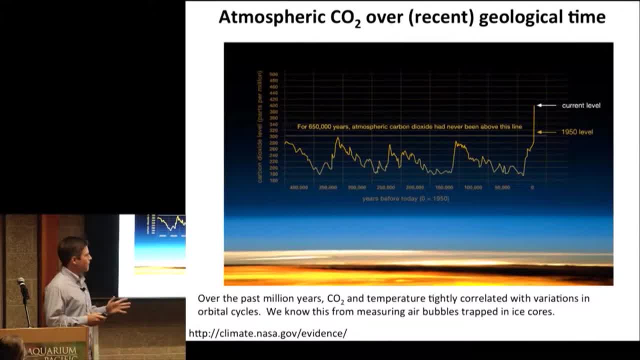 are so concerned about adding CO2 to the atmosphere, we start to think about geological time, And so if you go back 500 or 1,000 or a million years and look in the ice cores, you can find these oscillations that are due to the orbital variability. 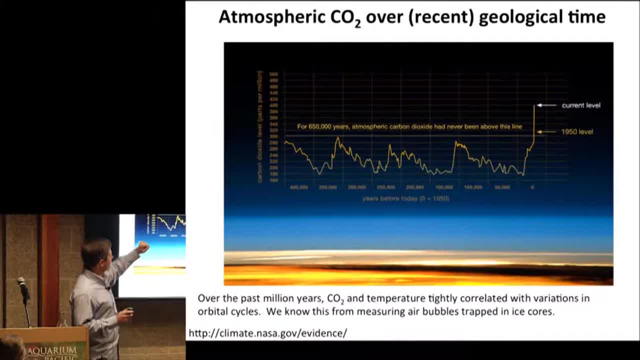 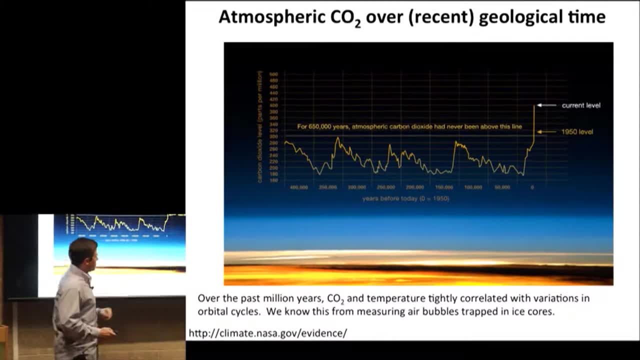 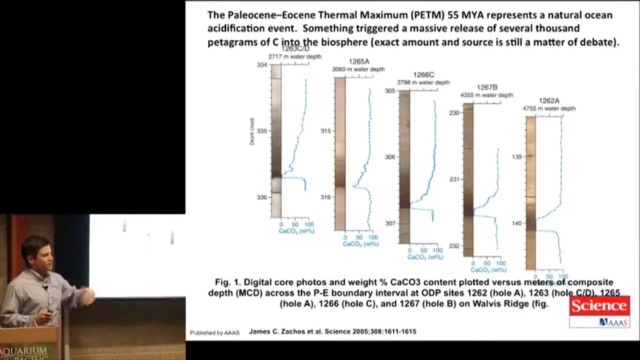 of the sun. Orbital variability of the Earth around the sun causes these Milankovitch cycles And we know that we've added this amount of CO2 and we're outside of this range over the last million years. And what's really scary is when you go back even further. 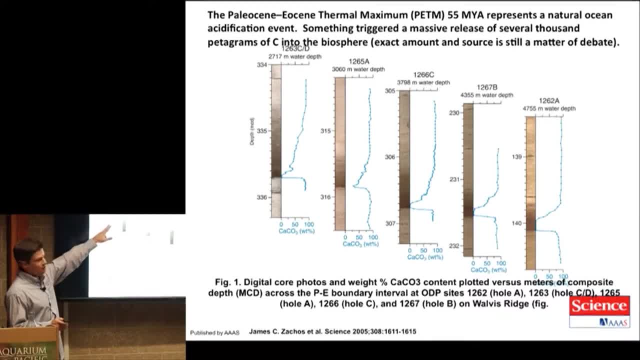 and you look at an extinction event 55 million years ago. for example, we call this the PETM, looking in cores, in sediment cores. there's this really stark transition that happened, which was some type of an extinction event at 55 million years. 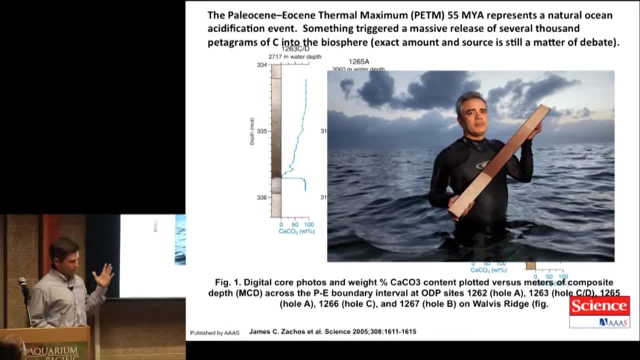 And just for dramatic effect, here's the author of the science paper in his wetsuit holding the core. I guess he dove down and got the core at the bottom of the ocean, I don't know. So Jim Zakos dove to 2,000 meters and cored that thing. 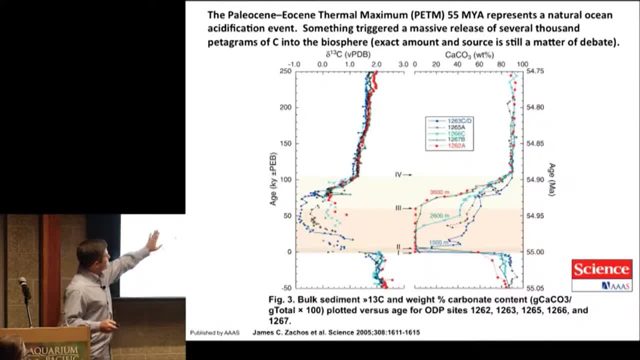 And what this tells us is that we look at two different things in these cores. but this term, that says del C-13, is telling us something we think about and a huge input of, maybe organic carbon into the biosphere, And that would be analogous to burning a lot of fossil fuel. 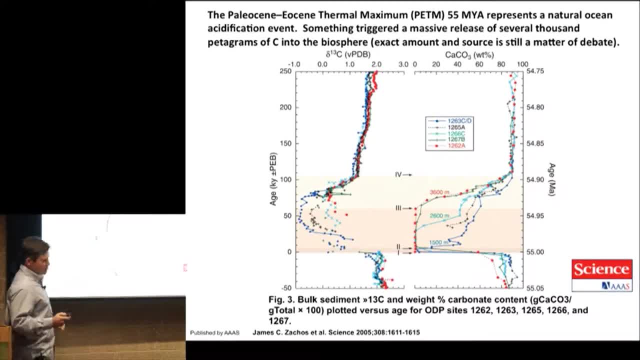 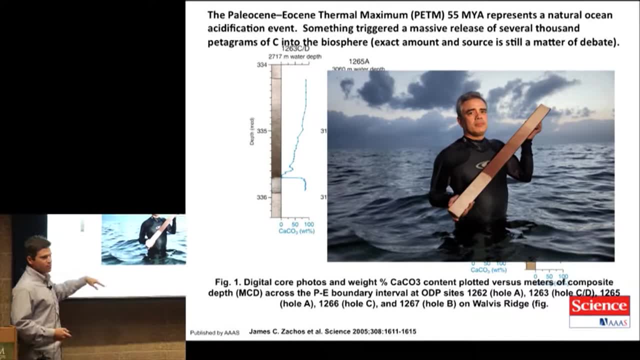 And what this shows is calcium carbonate weight percent in the core. So if you look at that, there's a bunch of calcium carbonate in this core and then there's none And it just goes away. And that's what's happening right here. 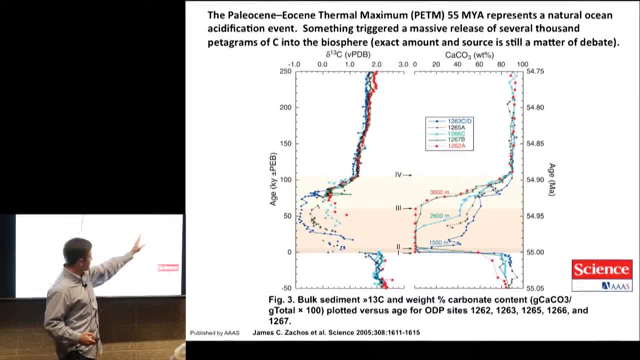 You've got going from 80%, 90%, maybe close to 100% calcium carbonate boom and it's all gone And it takes something like I don't know 100,000 years to get back to normal. And this event seems to be sort of what's happening now. 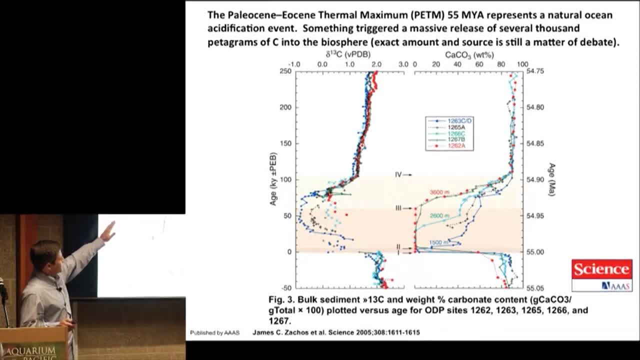 We don't know exactly how much was put into the atmosphere to do this. I actually just saw in Nature or Science there was a paper that came out last month with the co-authors at Scripps saying that they think maybe as much as I said- several thousand did I say that here? 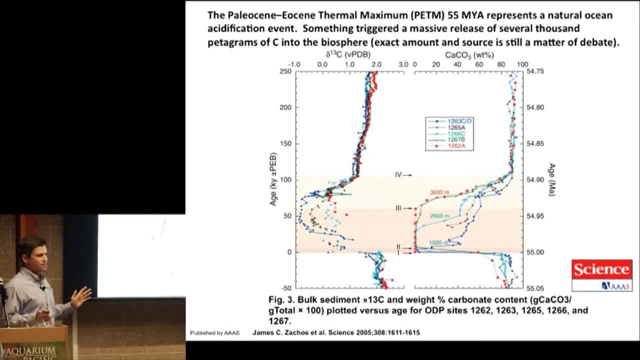 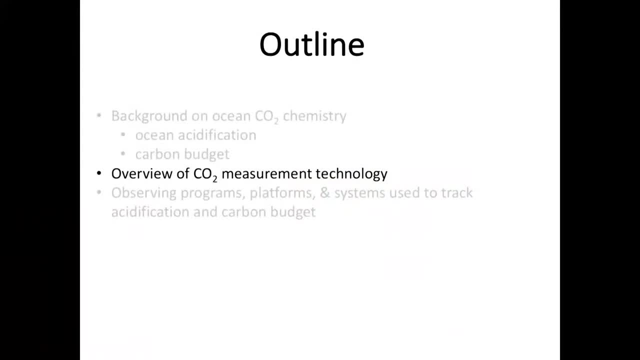 Several thousand petagrams. they think maybe 10,000. But the point is we put in something like 600, we're on our way. So big shift now. So that was just some background on carbon budget and ocean acidification things that I find interesting to try. 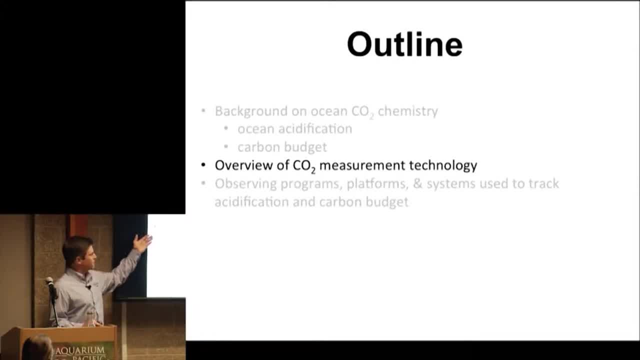 to set the stage for why we spend so much time working on measuring it well and developing new technologies to track CO2.. And so this is the. I'm going to maybe show a couple of things from my own work, But I tried to throw in some slides. 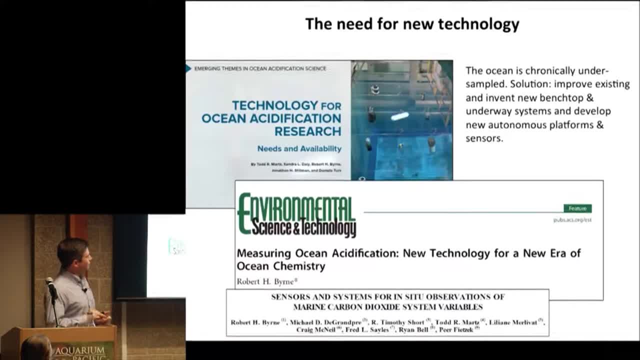 from my colleagues and various other people. So why do we need new technology? The ocean is chronically under sampled. We need to both improve existing technology, like what we're already using in bench top and under way systems. I'll explain those in a minute. 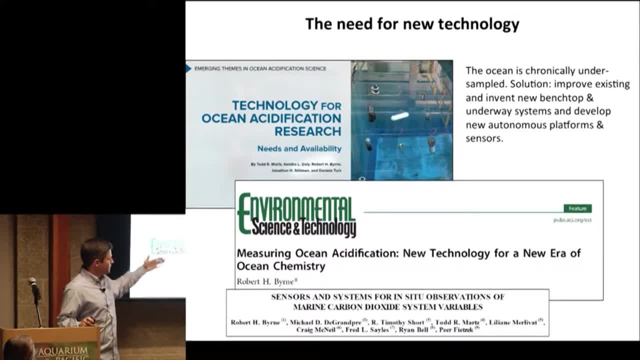 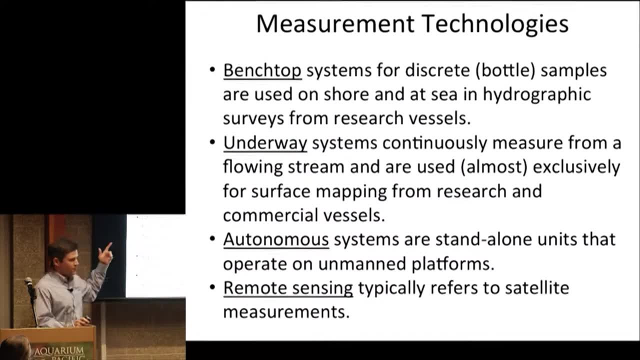 We also need to develop new autonomous platforms and sensors. This has been discussed by myself and several other people in recent articles. I've been doing this with a number of other people in the industry and I've been doing this with other individuals over the years. 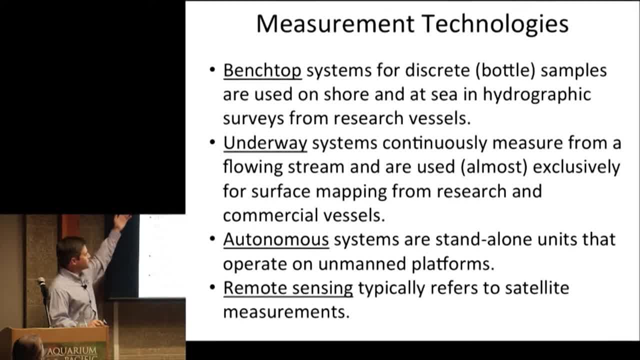 I want to just give a few definitions. As I talk about these instruments, I like to categorize them as bench top, which would mean things where I get a bottle of sea water, I bring it to my lab. I make a measurement on the bench top. 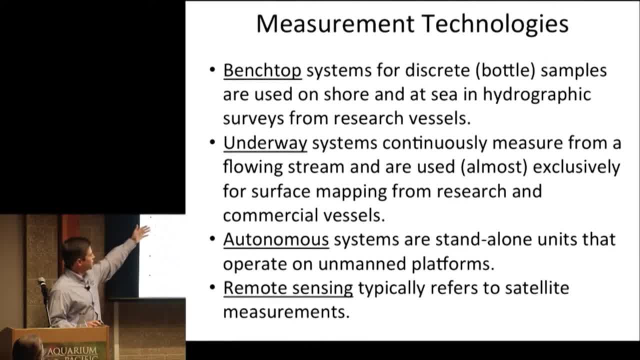 using some kind of system that's in the lab or maybe on a research vessel Under way, is automated. So you're on a research vessel, probably, or maybe a shore station, but you're pulling water in, you're pumping water in and it's continuously measuring. 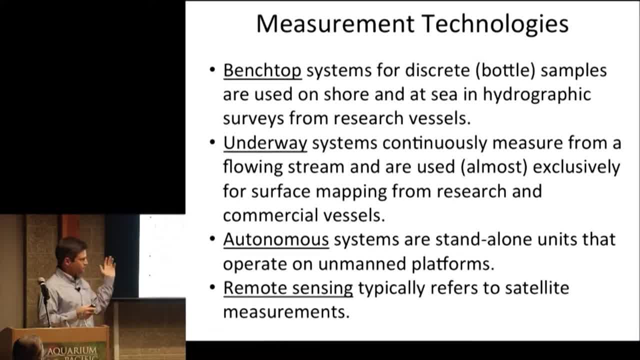 and it's generating a lot of energy. You're generating data, sending the data somewhere, logging it. You're getting a continuous stream of under way data, probably from a moving platform. Autonomous systems are completely stand alone. They have a computer that's logging the data. 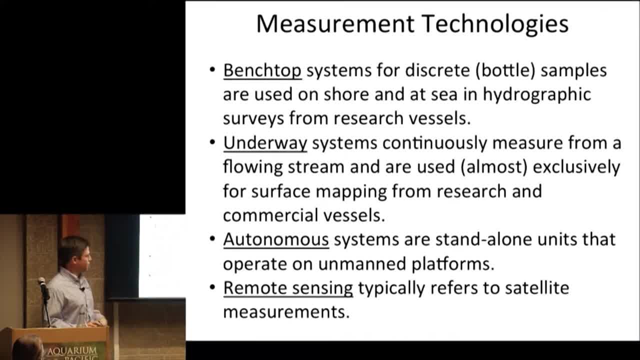 There's no human operator involved And they're on some type of a totally autonomous platform is my definition. So that would be like a buoy or something in the ocean, And sometimes people get remote sensing confused. but when I say remote sensing I'm talking about 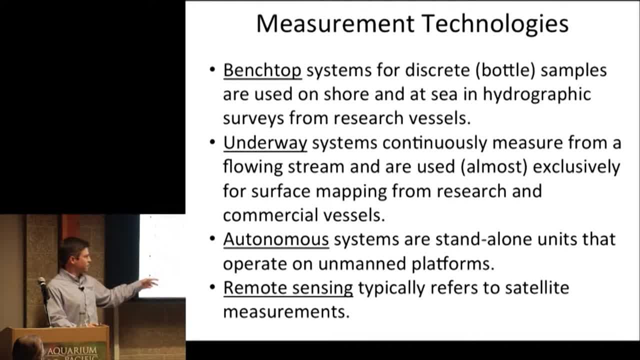 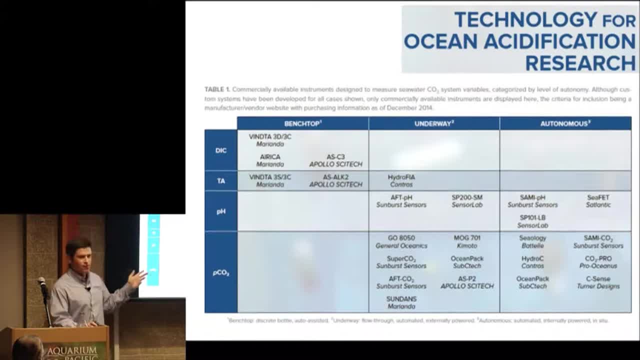 satellite measurements. Satellite measurements, Satellite measurements. This is from a paper that I wrote a couple years ago that categorizes. Remember, I said there's these four master variables, the measurable things of the CO2 system, and I've screwed up because I've written DIC. 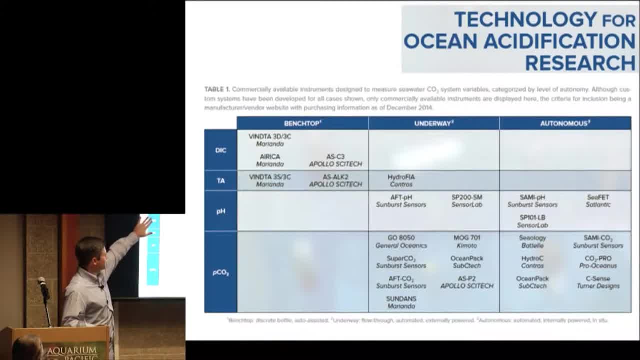 instead of C sub T, but this is the total amount of carbon, total alkalinity or the carbonate alkalinity, pH and partial pressure of CO2, categorized by level of autonomy. And one thing that jumps out is that not all these boxes are filled. 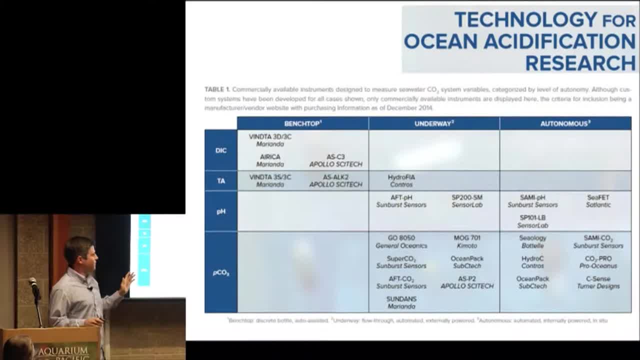 If some of my courses, if my colleagues, were here, they'd be very quick to point out that people have published papers in every box here for sure. What I'm showing is what's commercially available, So this is what people are pretty much restricted to. 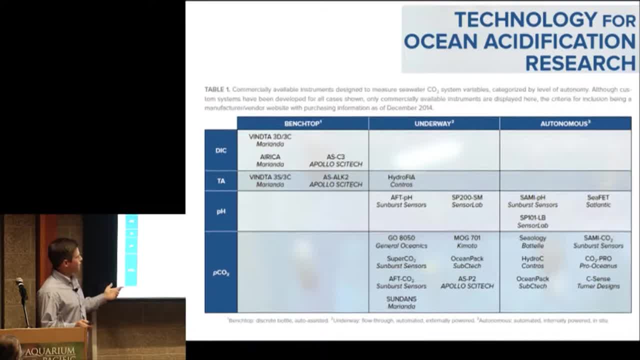 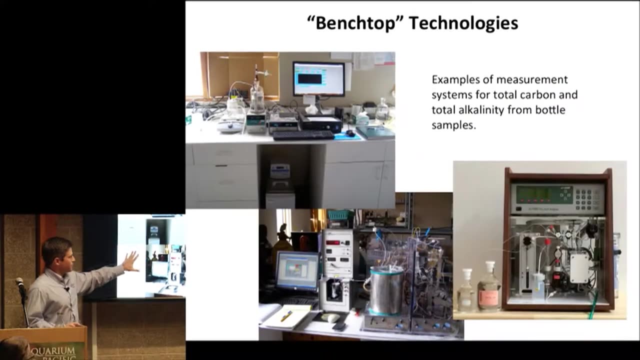 nowadays for observing the CO2 system in the ocean, And these boxes that are unfilled are things that people like myself are working on. We'd love to build an autonomous dissolved inorganic carbon measurement on an autonomous platform. This is the type of instruments 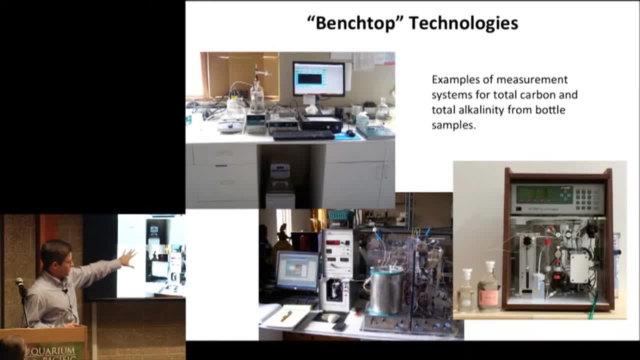 that I'm talking about, that sit in my lab and other people's labs. This is Andrew Dixon's lab at Scripps. This is a titration system used to measure total alkalinity. This apparatus does the DIC or the C sub T. 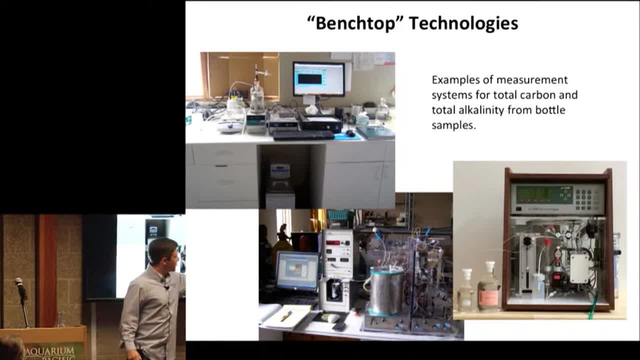 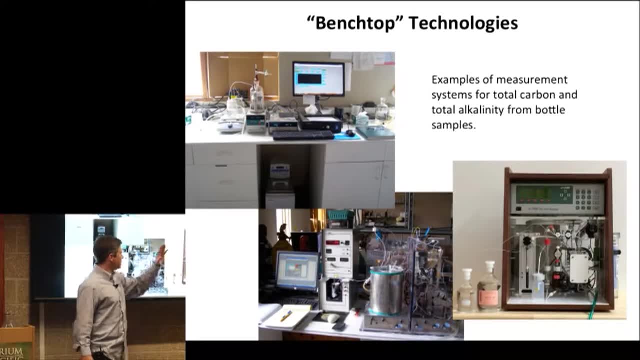 the total amount of inorganic carbon in the sample. And this actually does the same measurement as this, except it uses a different detection scheme at the end. So this is an infrared gas detector. that's called a coulometer, So kind of. 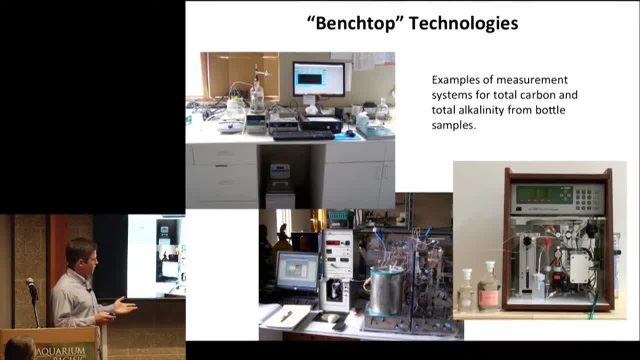 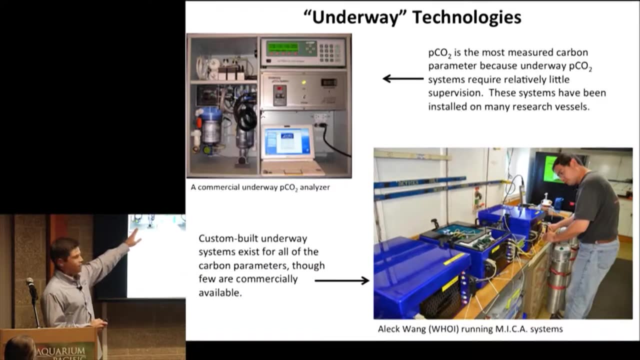 complicated systems, lots of tubes, lots of points of failure is the reason I'm showing this picture. They work when you have an expert operator. Very difficult to turn this into a completely under way or even an autonomous system. There are a lot of very successful 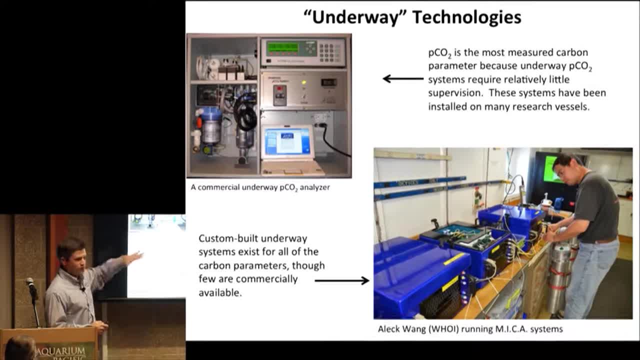 under way measurements that measure the partial pressure of CO2 all around the surface ocean, and that's because it turns out PCO2 is probably the easiest to measure. It's arguable: pH is pretty easy too, but PCO2 is one of the 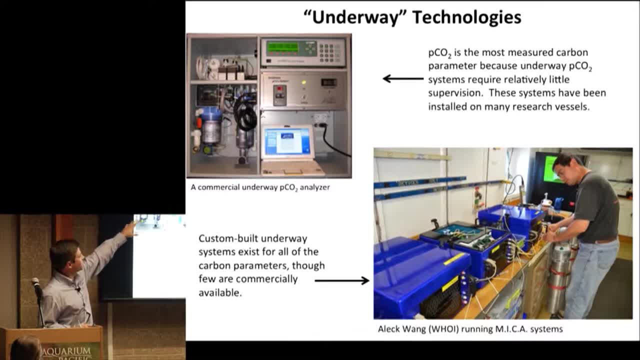 simpler measurements that you can make. You can set up a continuous flowing line with some kind of an air gas liquid equilibrator and a detector and you're on your way and you're making under way measurements. My friend, Alex Wang, has built very more complicated. 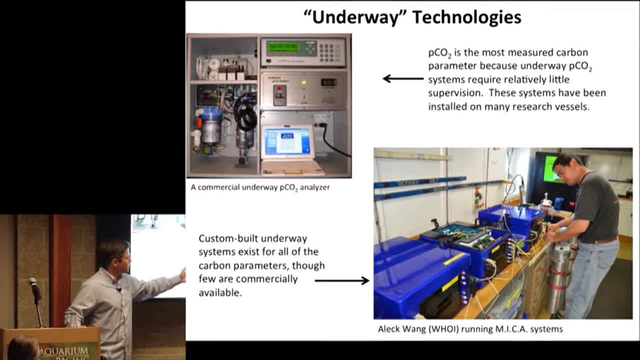 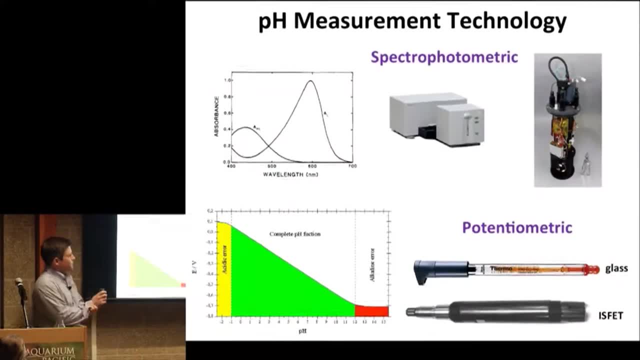 systems to measure other parameters of the system, like dissolved inorganic carbon. But, as you can see, it kind of takes Alex to run it. It's more complicated. This is a little bit more in my realm. I've done some work with pH. 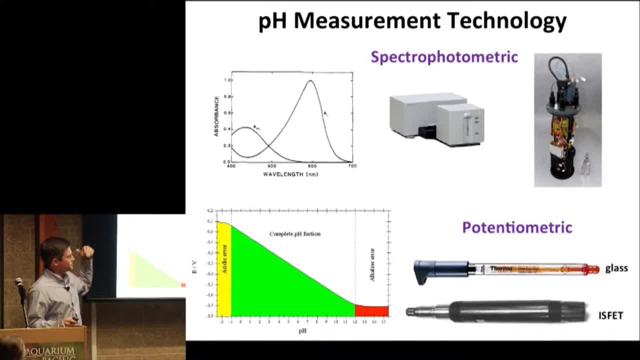 sensors actually in both of these areas. but pH is. it seems like it's an easy measurement to make but there are some pitfalls that people can make. But this is really divided into two different types of instruments that are either spectrophotometric- so if you 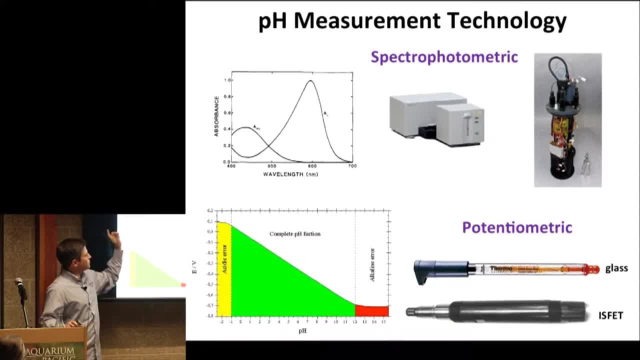 think about litmus paper that we use to measure pH. what marine chemists do is they take the chemical on the litmus paper and they dissolve it in water. they put a little bit in sea water and then they put it in a spectrophotometer. 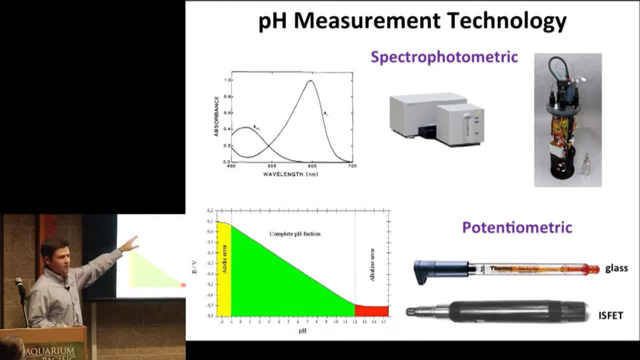 that measures the absorbent spectrum. You can get repeatable measurements into the fourth decimal place. with this It's the gold standard for pH measurement, Like .0004 pH unit resolution. It's amazing. You can actually do really well with potentiometry, which is even simpler. 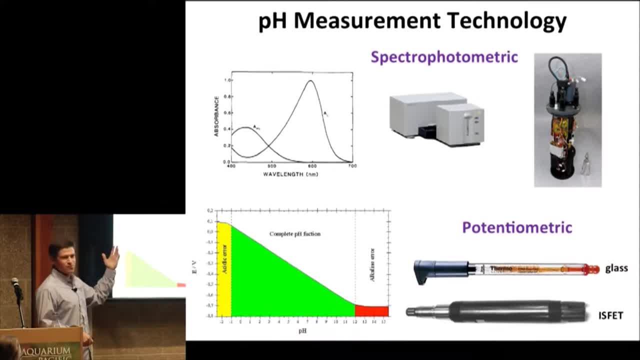 So a glass electrode you literally just put in your sample and it gives you back a number. Does it always give you the same number? Does it drift? So we have to worry about things like instrumental drift a little bit more in these, And I'm going to show you a few more slides. 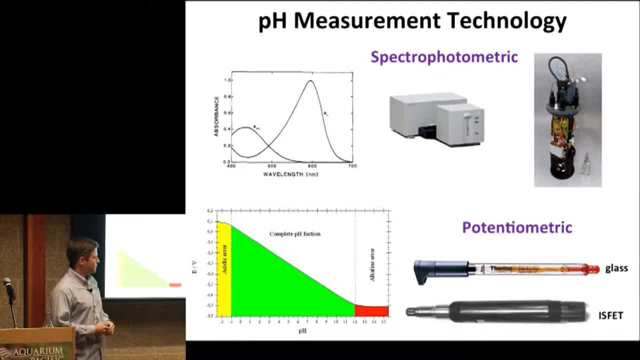 talking about this ISFET technology, which is one thing that my lab has focused on in recent years. It is a nice simple measurement because you just have pH and you have a voltage that comes out And usually you can make it a really 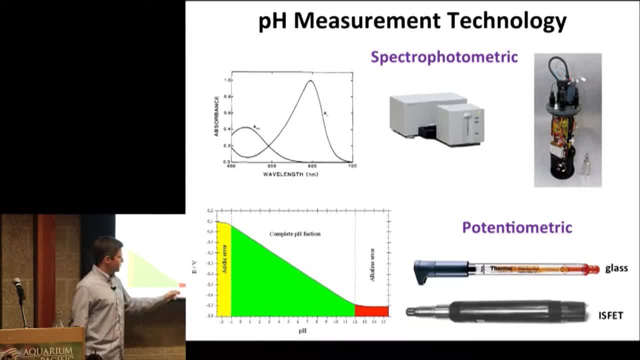 straight line if you understand some of the nuances of how the sensors work. This ISFET stands for Ion Sensitive Field Effect Transistor. It's a technology that was developed in the late 1970s, and Honeywell really pushed it to a high level. 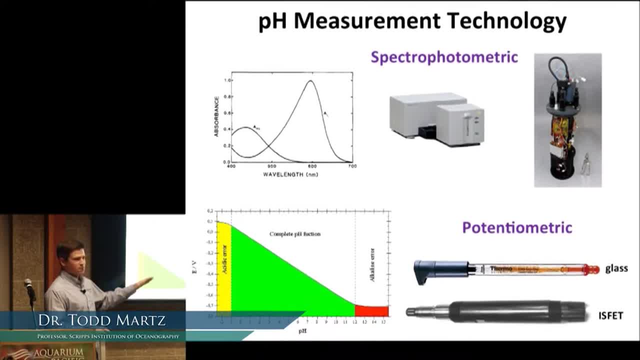 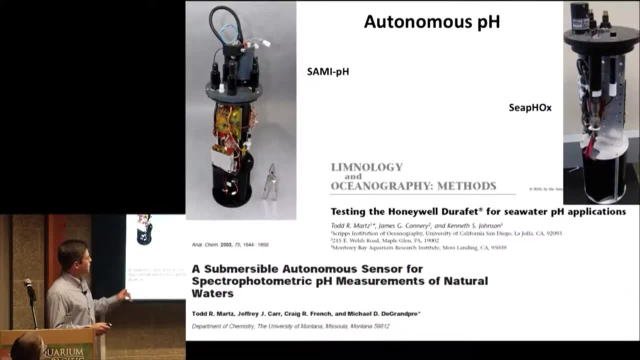 of operation, and it's replaced the glass electrode in many laboratories and industrial settings, And so we had adopted this and started to put it in seawater. I had the good luck to work on a spectrophotometric autonomous sensor as a graduate student, which was 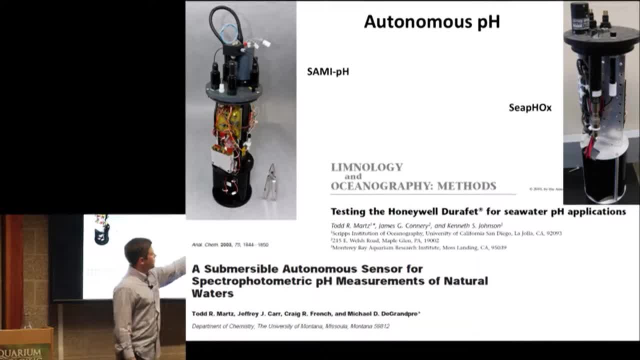 this paper back in 2003, and then move over and start working on the Ion Sensitive Field Effect Transistor we called so. the SAMI is the Submersible Autonomous Morse Instrument for pH, and we call this the CFOX because it measures. 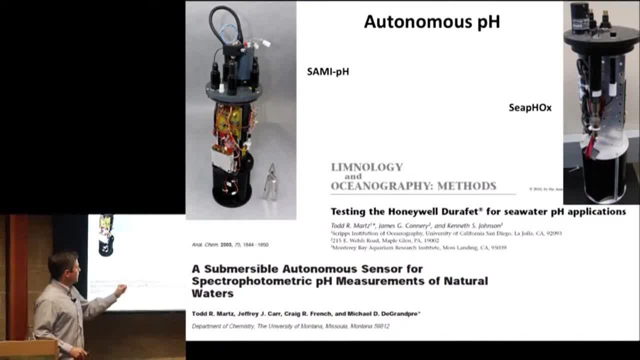 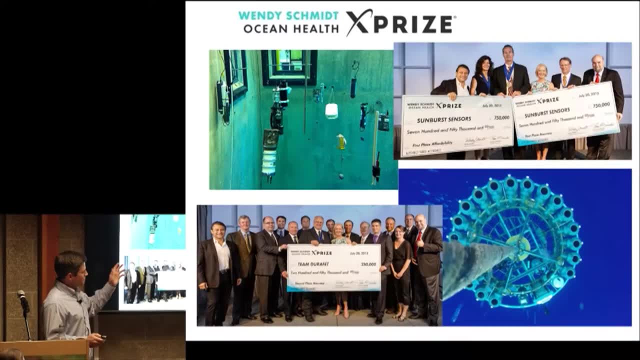 I guess pH and oxygen. we have an oxygen sensor in there. But I worked on these two papers so I kind of did both ends of the pH measurement thing and we ended up, like Jerry mentioned, we ended up competing those two against each other in the X Prize. 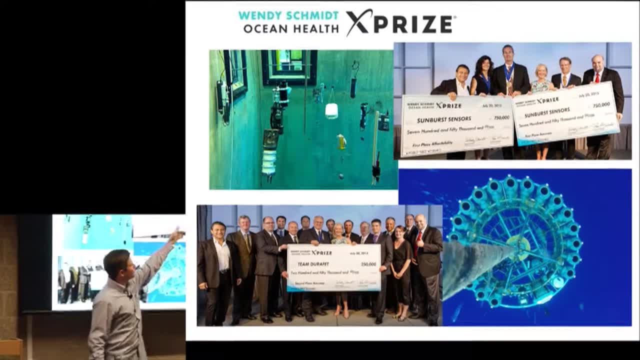 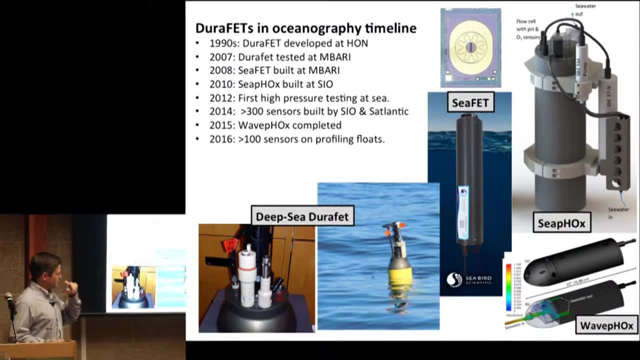 And my graduate advisor, Mike DeGrandpre, won the X Prize and we took second with the ISFET sensor. But these ISFETs have been really useful in a variety of different designs because they're so low power, easy. it's a solid state sensor. no. 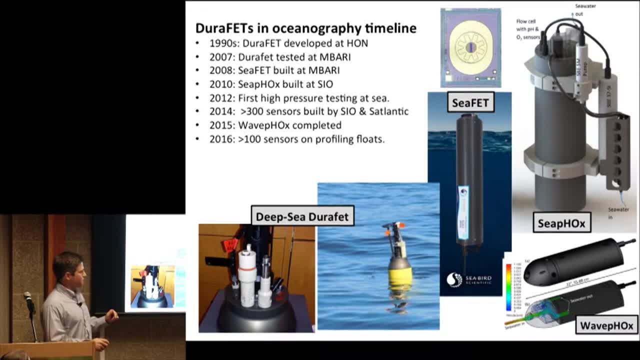 moving parts, pumps and valves and all that. So it has really been latched onto by the oceanography community. We've now put them in a variety of different packages, And this picture at the top is the chip itself. it's about 2 by 3. 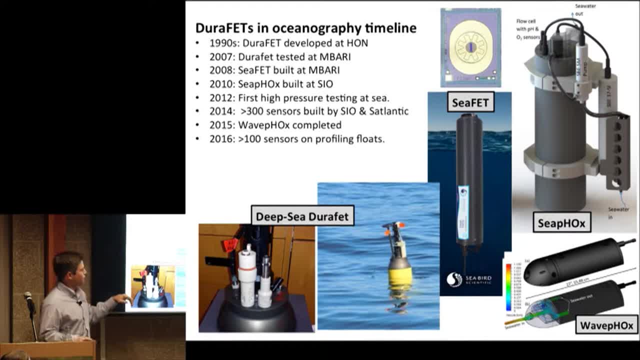 millimeters, And this is just kind of the history of where those are. now They're commercialized and they're selling hundreds at Seabird. We've built weird designs and tried to put them on stand up paddle boards. This is the one that I'm going to talk. 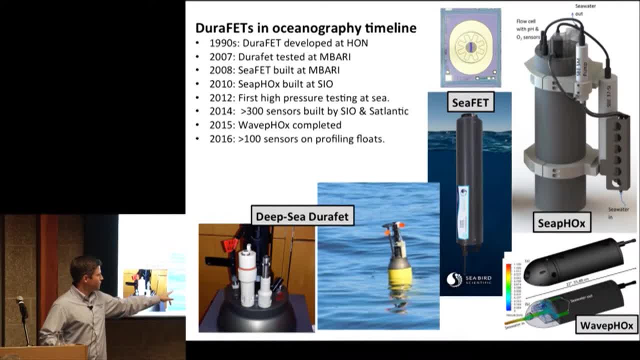 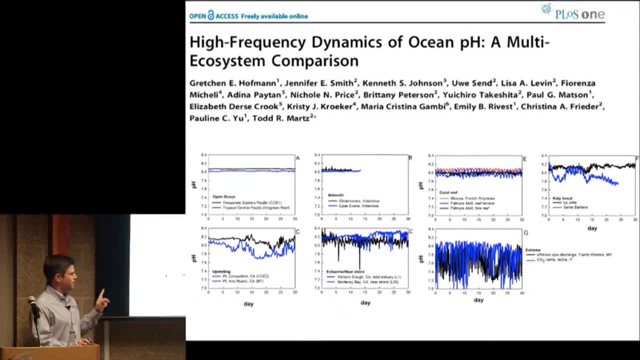 to you a little bit more about in this talk, which is the version that's on profiling floats. We call that the deep sea durafet. But first I'm just going to show you one slide on kind of the history of those early pH measurements with the durafet. 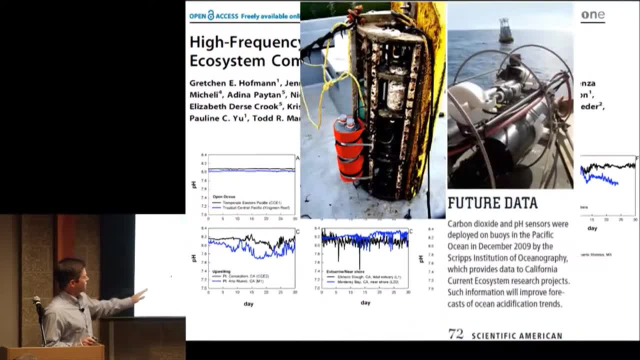 and Jen may talk about this a little bit later, but we started putting these around various sites in the open ocean, where pH is very stable, And then in upwelling zones along California where you see much greater excursions in pH, And estuaries also, where you see. 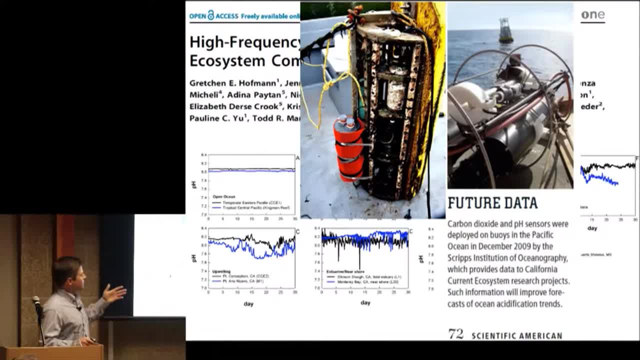 more like tidal fluctuations in pH, And so this, these early measurements were really we already kind of knew this, but this paper was one of the first ones to kind of document all these different settings in the ocean with kind of simple, same scale, 30 day snapshots. 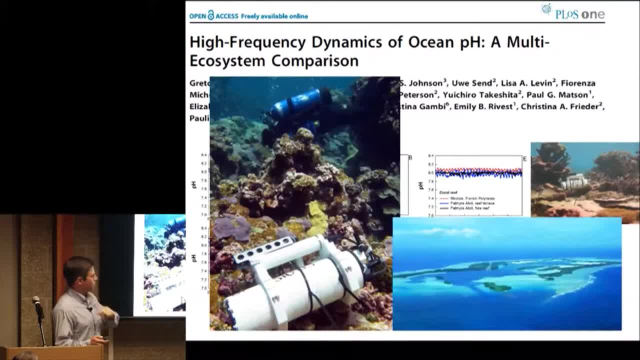 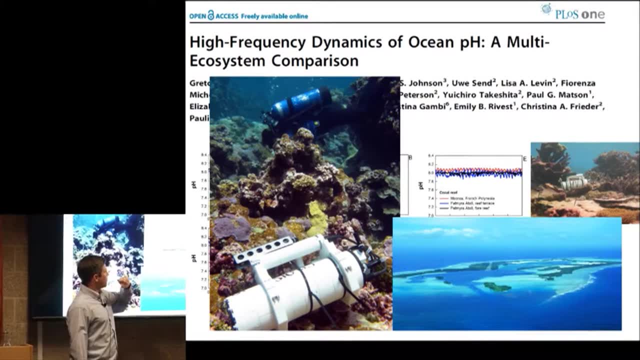 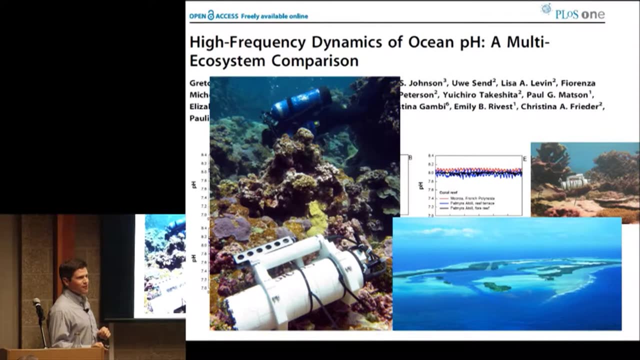 of pH. We had put them, worked with Jen to put them on coral reefs and those went to Palmyra and Morea and the pH patterns look much different there. There's kind of more of a daily pattern, not the negative excursions. 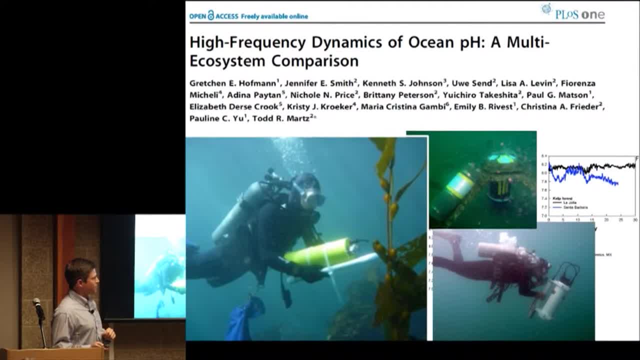 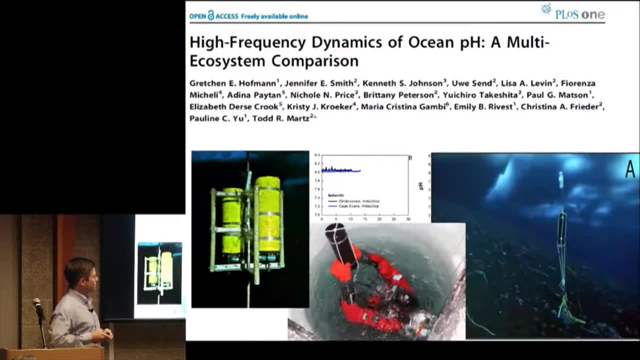 Some kelp forests along the California coast and Santa Barbara and La Jolla, And we also- this is my favorite- was Antarctica work. Fortunately I didn't get to do that, but they have even put these things underneath moving ice sheets in Antarctica, and there are. this was 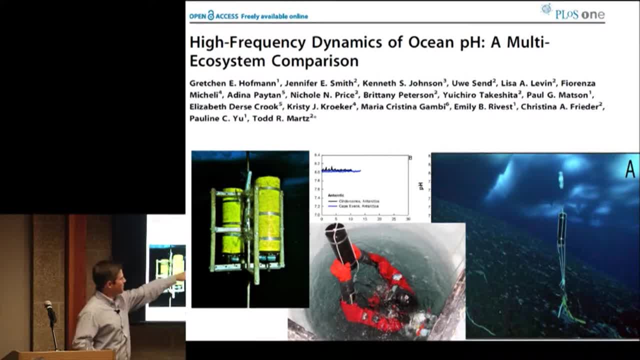 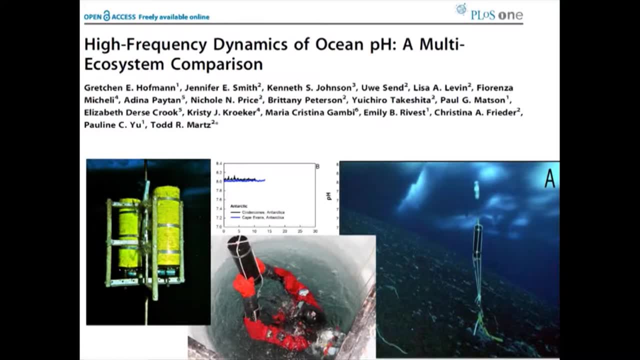 the very early data set. We were excited to get the paper out, so we only had like 15 days of data, but since that we actually had. this is Gretchen Hoffman up at Santa Barbara- her group's work. they've gone back and captured entire years. 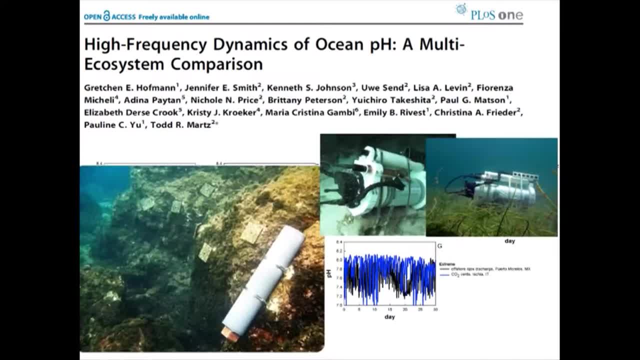 and we've even captured some under ice data from floats, And this is some really weird stuff. we call- I just labeled it- extreme, but that's like CO2 vents in Italy, and I think I have one more slide from that in here. And the last thing: 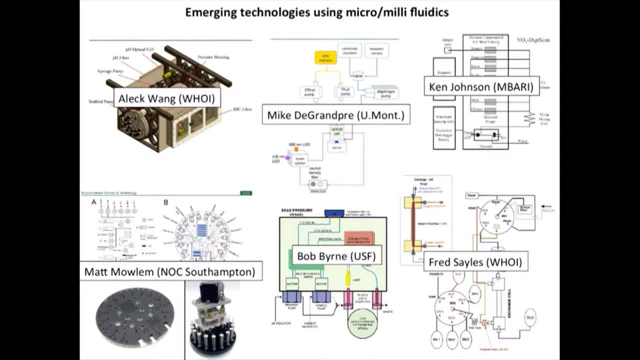 or I think I may have one more, but I want to just mention that, in terms of emerging technologies, beyond these pH sensors that I just showed you, there are a variety of people, and myself included. I didn't have room for myself in this slide. these are some of my colleagues. 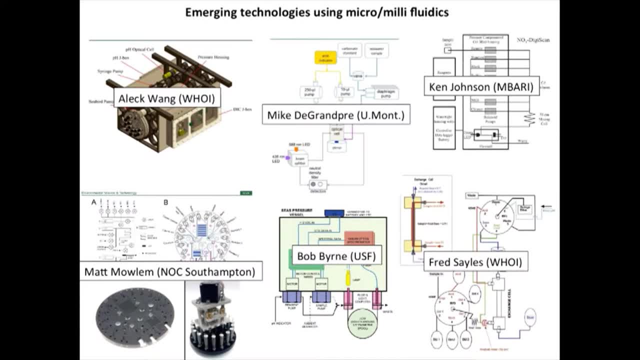 People are working on much more complicated things, kind of in the micro millifluidics realm, to try to expand the measurement suite beyond just the pH and the PCO2.. So we're talking about some fairly sophisticated engineering approaches to move fluids around through. 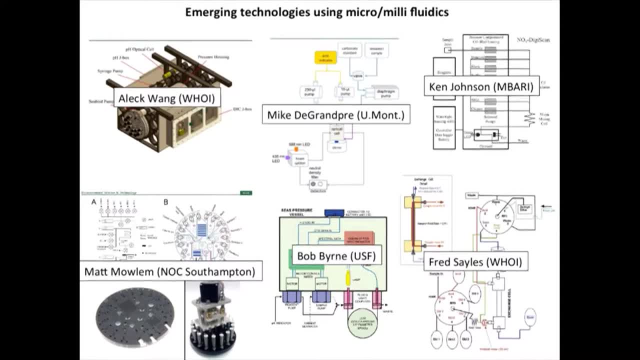 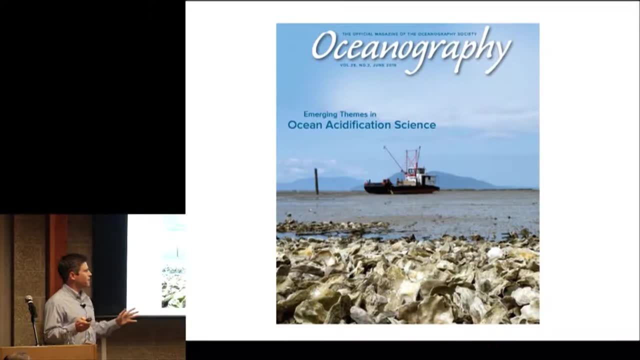 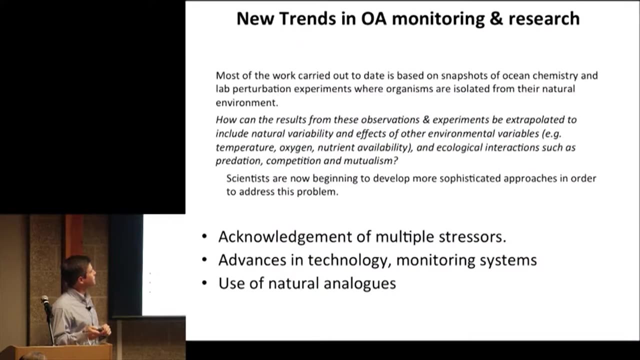 small manifolds and try to do bench top chemistry at a micro scale, And I had just thrown in a couple of slides on other emerging themes. This was from a special issue in Oceanography Magazine. Most of the work that I just talked about is 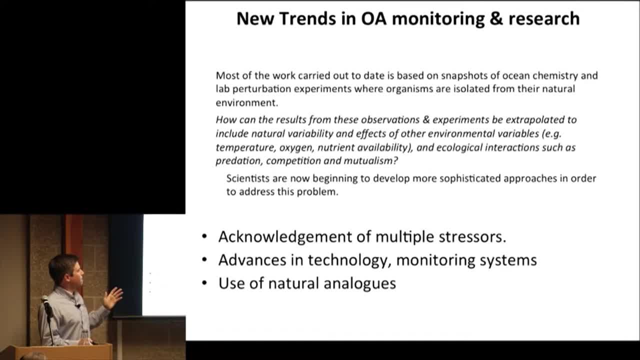 really snapshots of ocean chemistry. But what I think people like Jen are starting to think about is how can these observations of the ocean be put into context and tested? with more of a holistic view, People are beginning to acknowledge that it's not just the pH or the saturation. 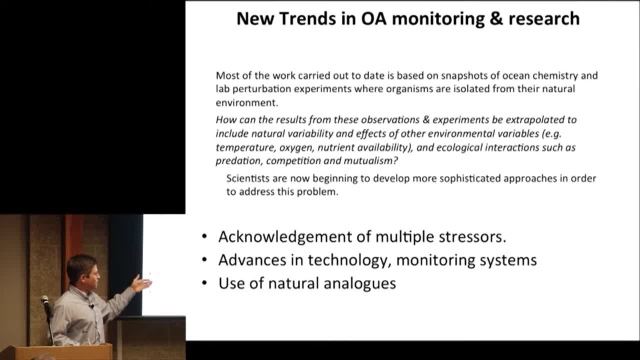 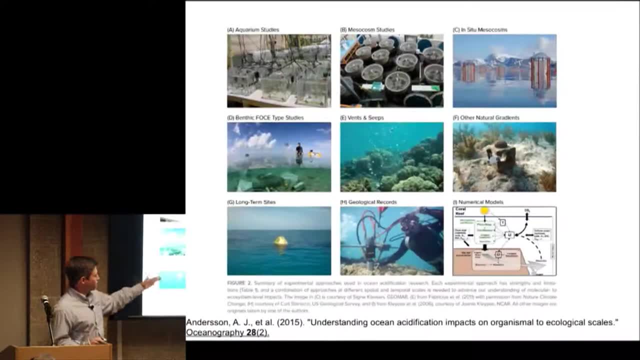 state, but there are multiple stressors that have to be taken into account. There are advances in technology and there are these natural analogs. So Andreas Anderson published a paper that kind of captures what I just had in that previous slide and showing where people are doing experiments. 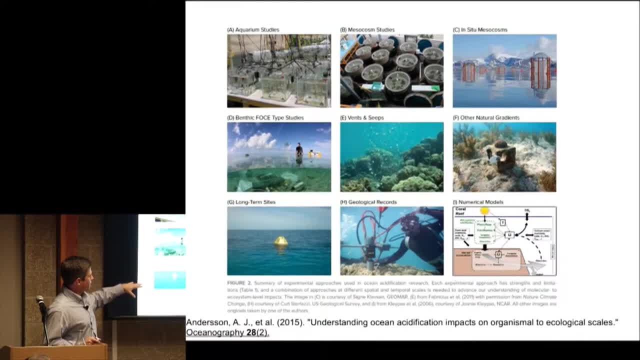 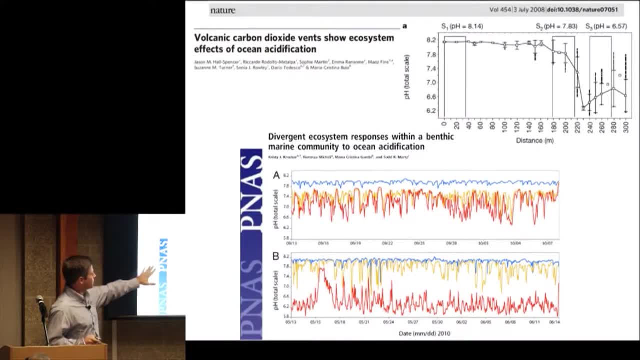 in the field of ocean acidification, kind of following that envelope to use these different, more holistic ideas, I guess. So this is just one example of using a natural CO2 vent as an analog for a high CO2 world. Christy Croker and. 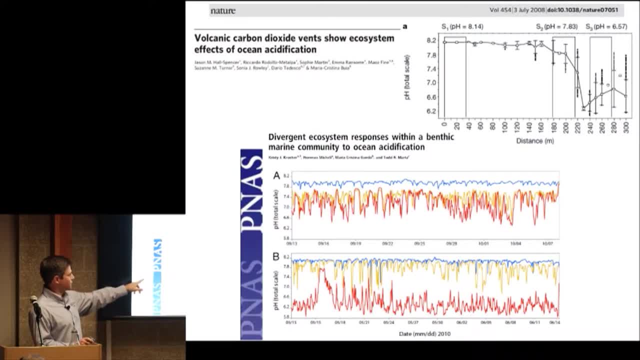 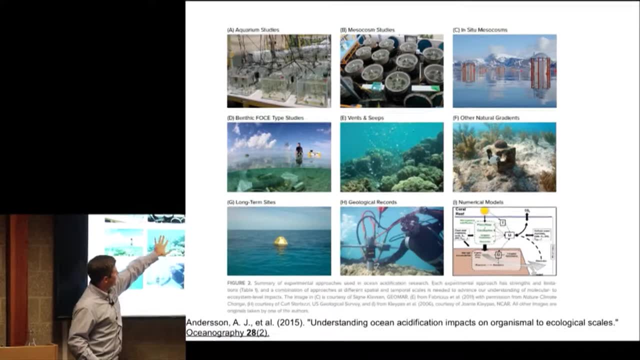 Theo Micheli at Stanford collected this with some sensors that we built. This is one of those weird CO2 vent sites where you have basically CO2 bubbles coming up. This is a picture in Andreas' paper, but you can get closer to the CO2 bubbles and you can. 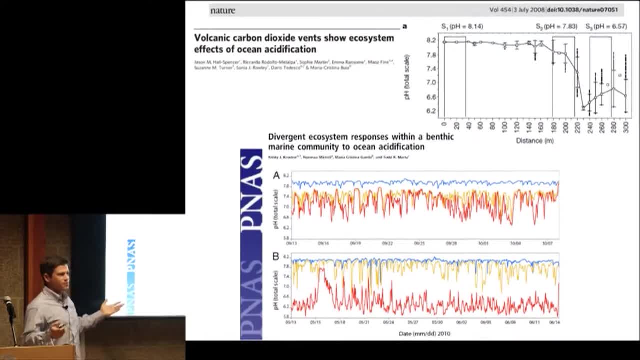 find a place where the pH is really low, that might represent something, say, 100 years out from now, and you could do experiments there. You can put out plants or something next to that and maybe gain some knowledge about how those organisms would behave in a future world. 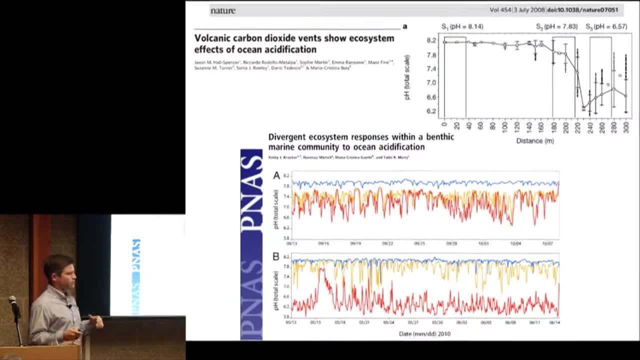 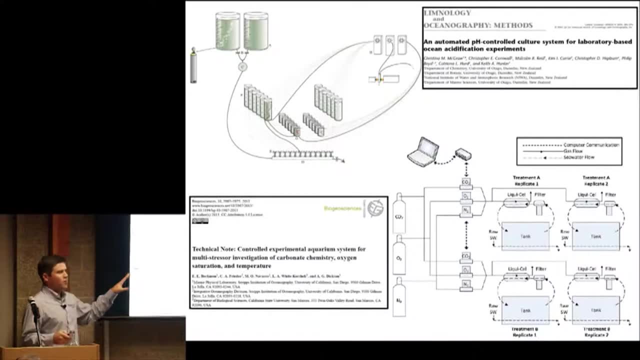 So we were involved in this just to the extent that we were helping with the sensors to get the measurements, but they did all the biology. And the other kind of emerging thing, I think, is that we're building more and more sophisticated laboratory control systems. 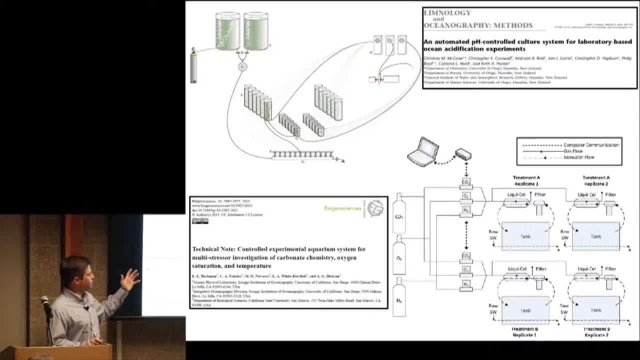 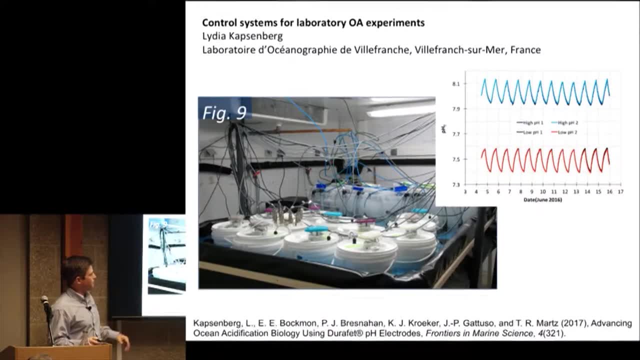 now to manipulate the CO2 chemistry so that we can test multiple stressors and test things like diel cycles. And this is just one example of Lydia Kapsenberg's work, who I've worked with, putting a bunch of sensors to control a multitude of aquariums. 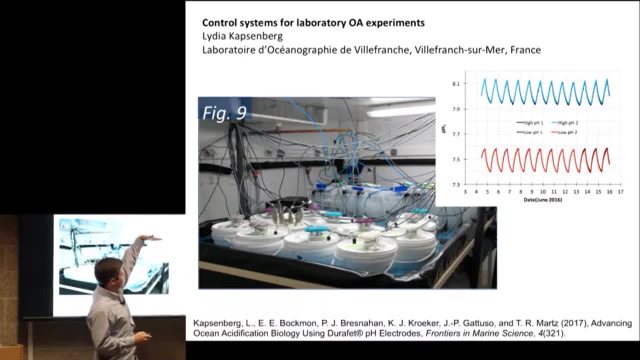 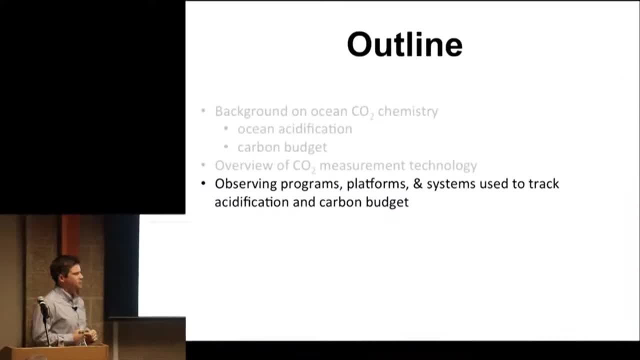 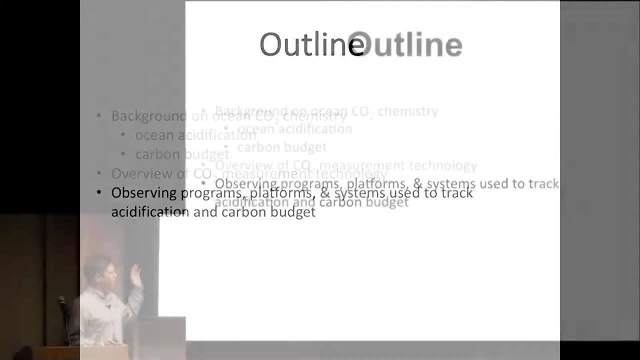 where she's growing something and then implementing things like a mean low and a mean high pH with some diel cycle. Alright, well, I have 15 minutes So I'm going to just talk as fast as possible. I'm going to try to. 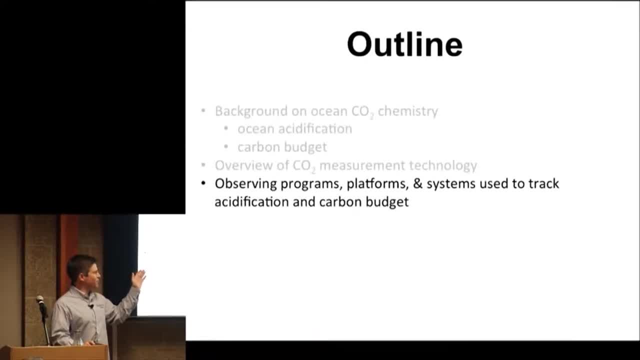 talk about. I'm just going to give an overview of some of the observing programs that have gone on in the past, and one thing I'm really excited about that just kind of found its way into this talk is the Argo observing system. This is the cartoon that 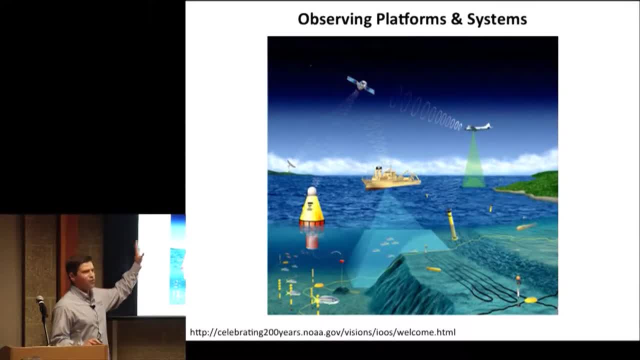 you may or may not have seen. that just kind of captures all of the different ways that we observe the earth, from the satellites to research vessels and moorings observatories at the bottom of the ocean, free drifting things like profiling floats, AUVs. 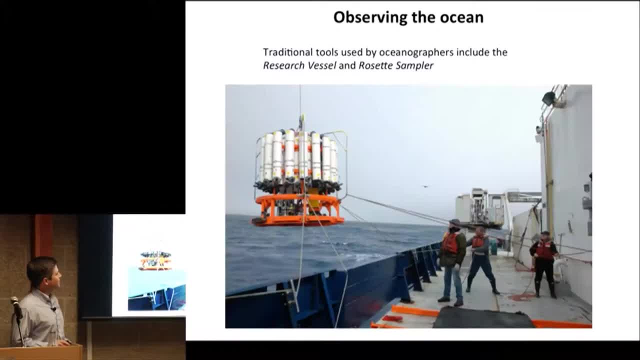 fish? I guess I don't know. This is the traditional tool that oceanographers have used. the research vessel that's this thing and the rosette sampler. You guys know what that is. Have you seen the rosette sampler? 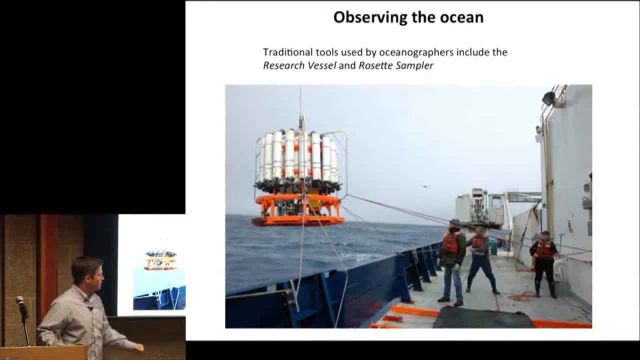 So this is a bunch of bottles. they cock them open and then they send that thing down on a winch and they close them at different depths, bring it back up on board. everybody goes around in a circle. they take samples off of it. 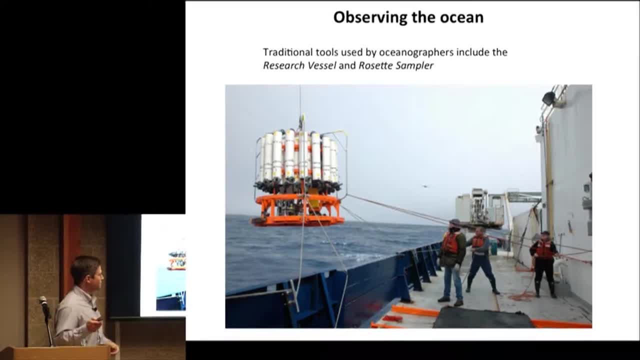 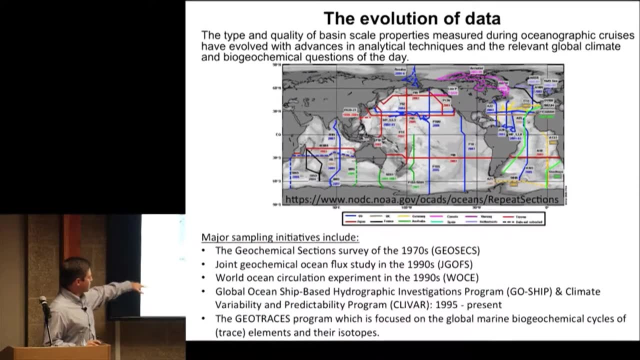 they go back to their labs and they measure it with their bench top measurement systems. So this is over the last 50 years. I'm only showing back to the 1970s in this, but we've been for about 50 years going. 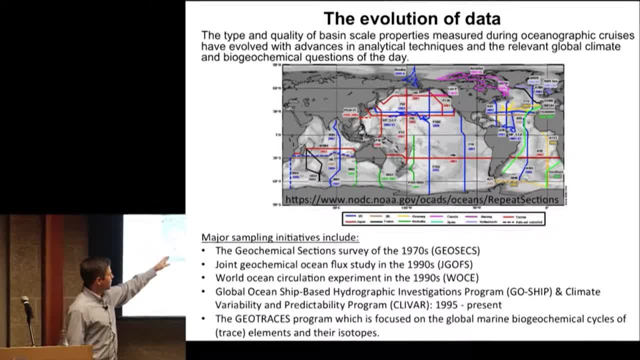 out on research vessels and doing a really good job of really accurate measurements along different lines in the ocean, approximately, maybe once a decade, so you might be at that particular station once a decade. This goes back to the GEOSEX study, followed by the JGOFS and the WOES in the 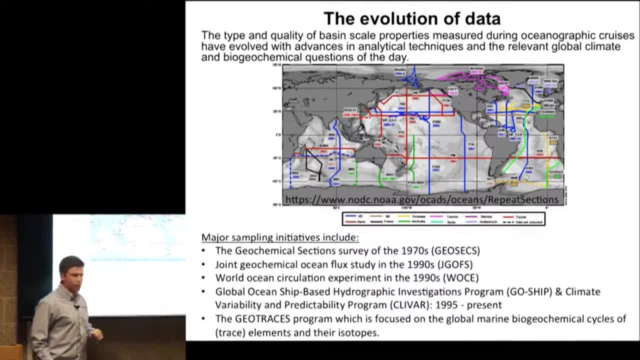 1990s. We have an ongoing program that's currently referred to as GO-SHIP. was the repeat hydrography program, now it's GO-SHIP, part of the CLIVAR program. lots of acronyms to process here, But the 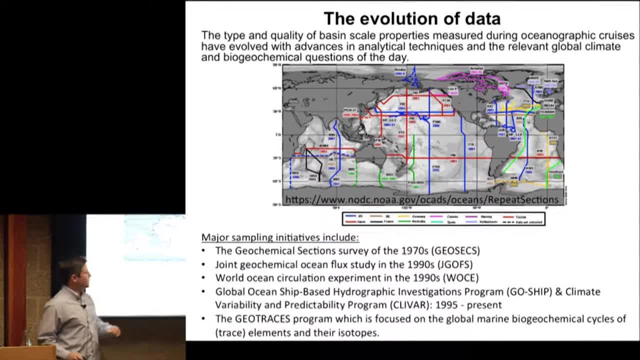 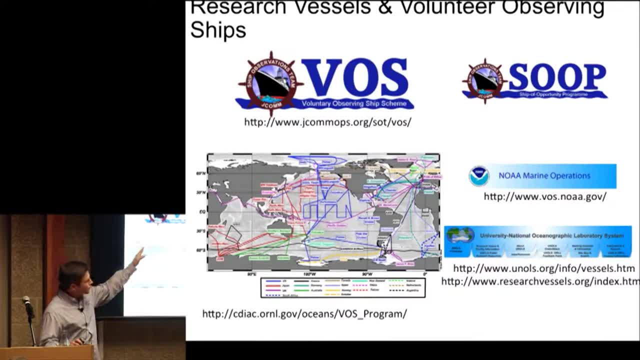 GO-SHIP program manages going out on these lines and sampling by ships. There are also what we call volunteer observing ships or, because we need two acronyms for the same thing- Ship of Opportunity Program, and these are on things like container ships. people go out and put 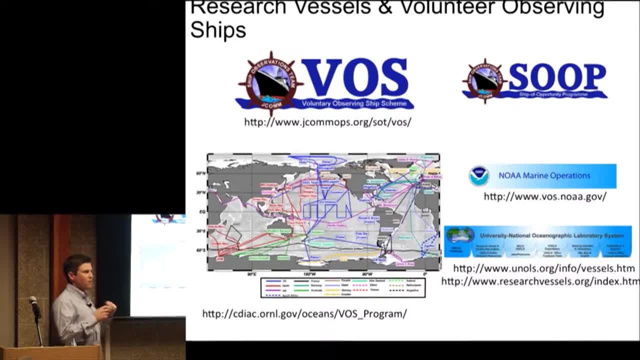 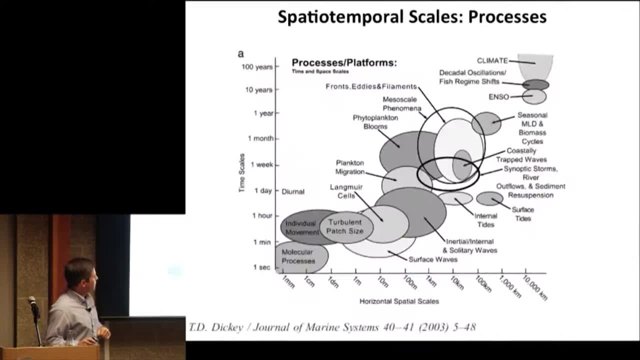 these underweight PCO2 systems that don't require a lot of maintenance and they're collecting CO2 data along these lines that container ships follow. So ocean geographers that are doing this type of work- and really any type of work- need to consider. 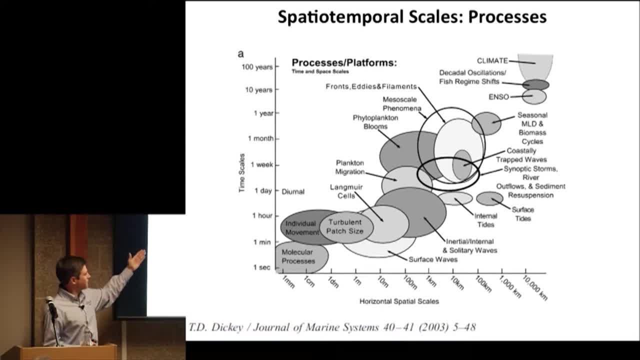 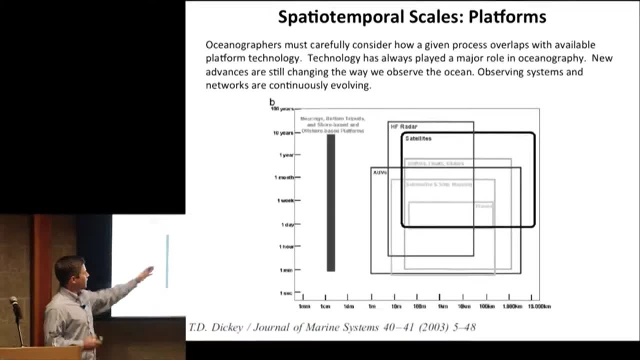 things like how the process of interest scales over time and space. So if you're interested in a phytoplankton bloom, what kind of a platform do you need in time and space to go observe that? Do you need to be on a? 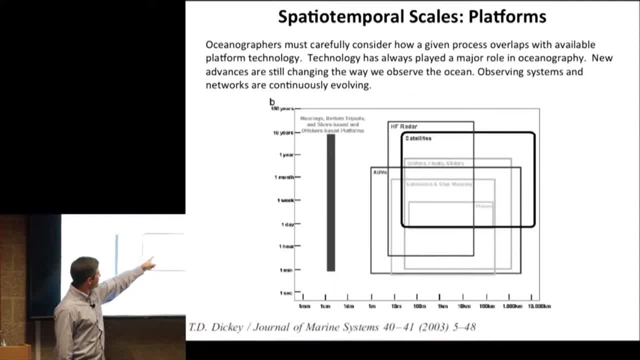 well, probably not a submarine. I don't know any oceanographers on submarines, but ships versus AUVs, versus moorings, are going to cover different time and space scales, So this is the type of thing that people that are interested in earth system observing. 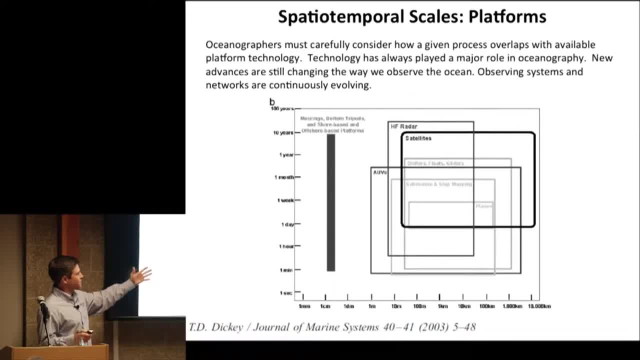 think a lot about is: can my system capture the process that I'm interested in studying? I said in this that technology is changing. observing systems are also continuously evolving. and one thing I'd say: just since 2003,, this line for floats and gliders. 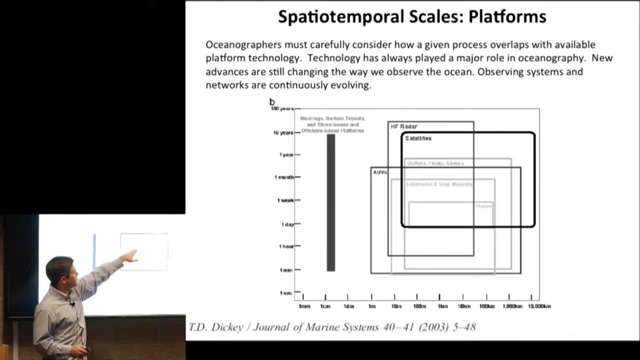 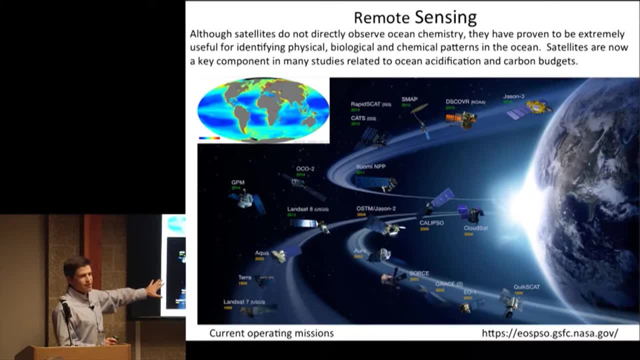 has to really be raised all the way up to satellites, because we've had float programs in the ocean now for a decade, so it is evolving And this one slide I'll show about satellites just to make note that they're very important even in ocean acidification. 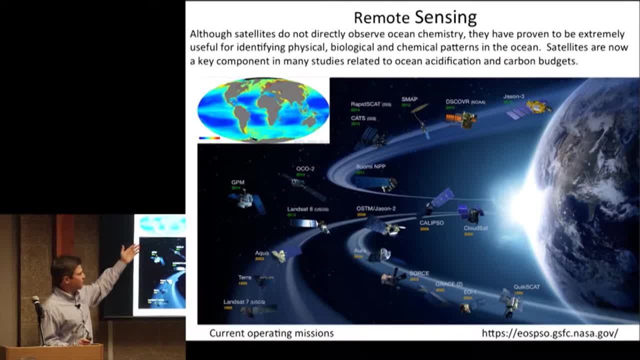 studies, not because we can directly observe chemistry from satellites, but we can observe ocean color beautifully and use that to coordinate with measurements in the ocean and try to expand them to a global scale. So satellites are extremely important to us in studying the earth system as a whole and trying to get 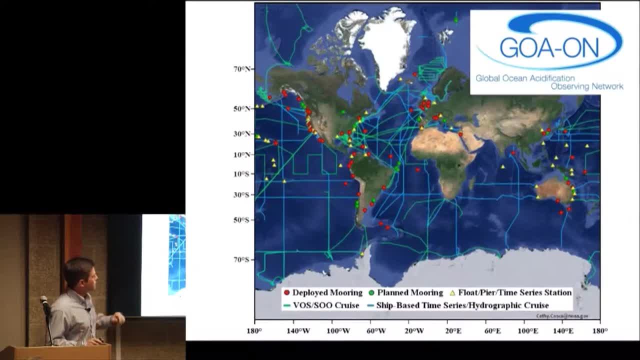 that to work together with the ship based measurements. This figure shows kind of all those, the two different types of repeat hydrography lines and the volunteer observing ship lines, along with a bunch of shore stations and moorings that all fall into what is known. 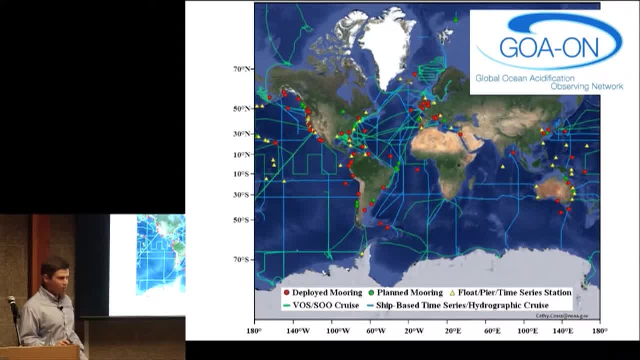 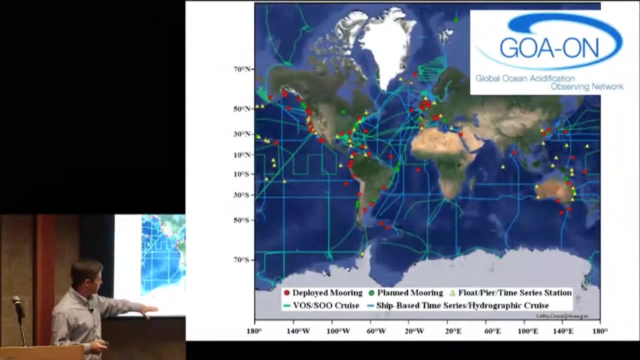 now as the global ocean acidification network or GOAN, And there are all sorts of different assets shown in this figure. The one that this figure contains is based upon just the VOS, the volunteer ship lines and the hydrography, So 50,. 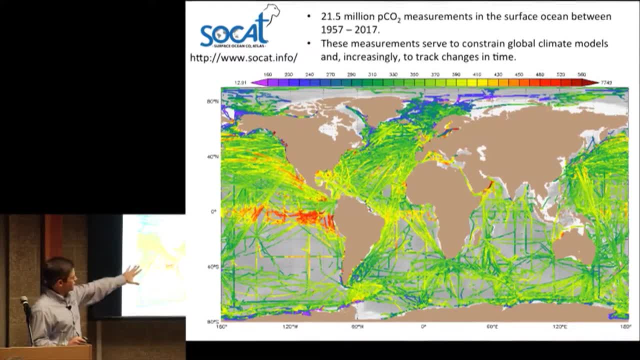 60, sorry, 60- years of data in PCO2 has generated an immense data set. 21.5 million PCO2 measurements have been made in the surface since 1957 that we have good confidence in And that's generated a 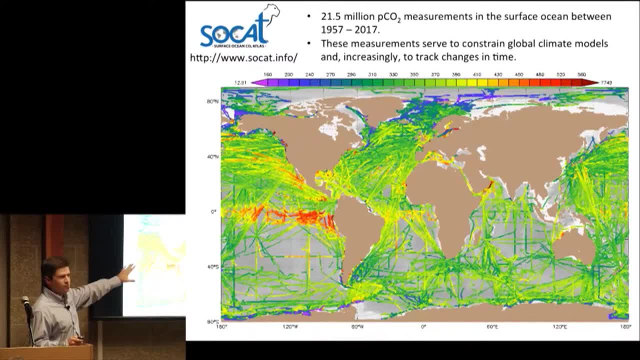 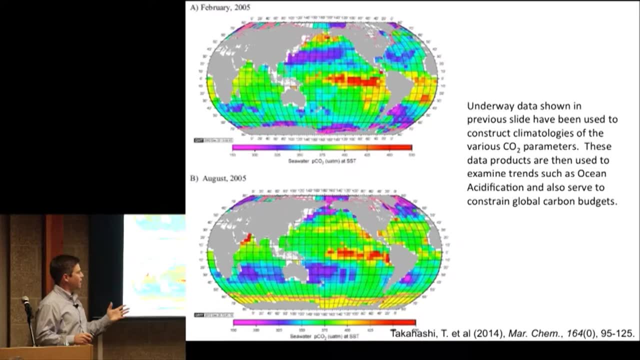 decent global picture on average of what the partial pressure of CO2 looks like in the ocean. This data set is compiled into seasonal averages. we call this a climatology, and data products are made to help us learn about how the different CO2 variables. 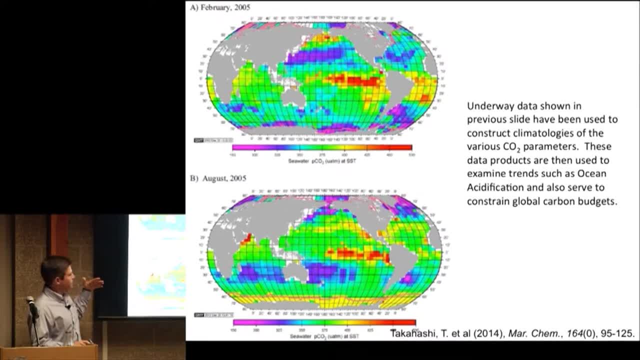 change throughout the year, say from February to August. This is just showing the seawater PCO2, which would reflect, if it's red, that that region of the ocean is actually a source to the atmosphere, versus a blue region which would be a sink. 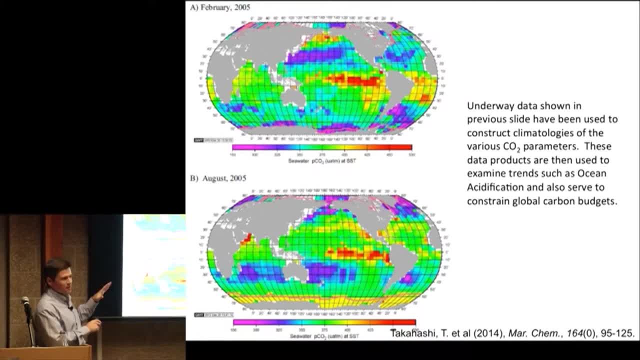 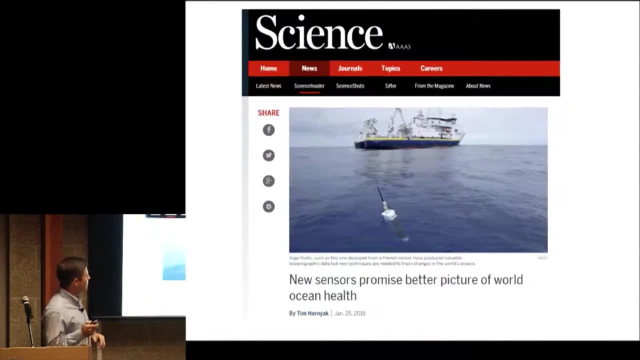 relative to the atmosphere. So it's a little bit more complicated in terms of just treating. we don't treat the whole ocean as a single source or sink. It begins to be a little bit nuanced. We're trying to. there are optimistic articles from time to time. 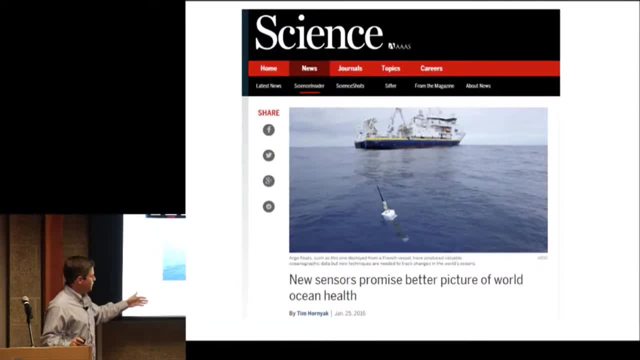 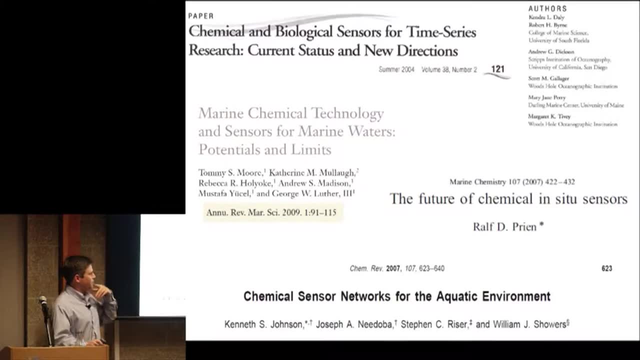 about how new sensors are going to solve this problem of under-sampling the ocean. Here's a recent one from 2016.. And I don't want to throw a wet blanket on it, but we've been saying this. actually, you can go back 10 years. 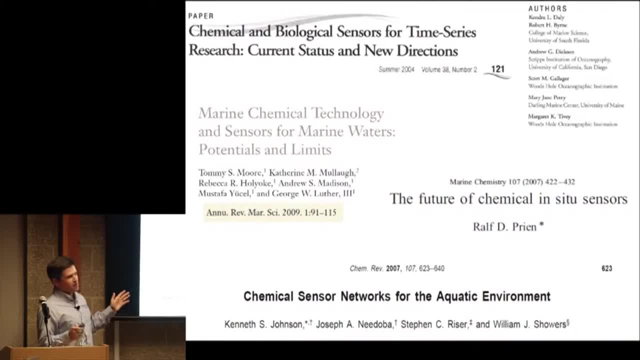 you can go back further, but the point here isn't that it's not possible to put new sensors out on these autonomous platforms, but it does take some time. So we've been working. I've been working on this in this field for over 15 years. 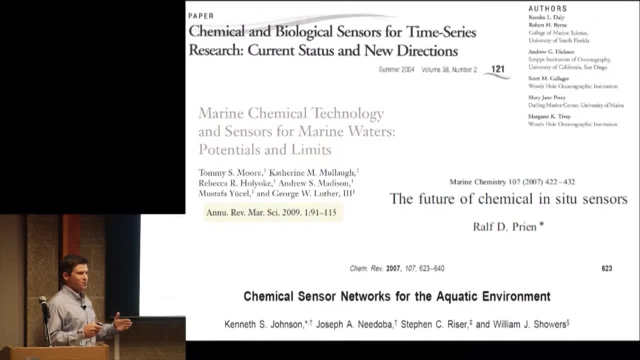 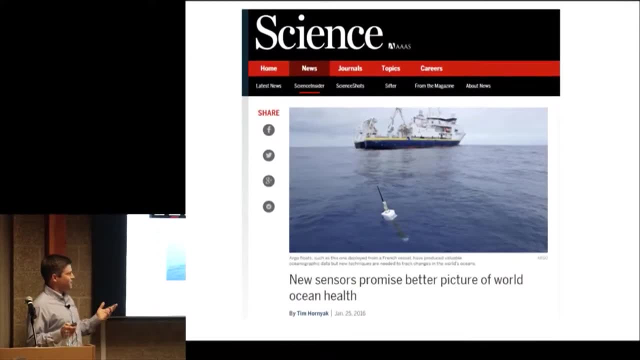 now and I've started to see that it's a very slow moving process to actually get the sensor from the lab out onto some system like that, But I'm still optimistic about it, And seeing the pH sensors get out on these types of platforms has really given me. 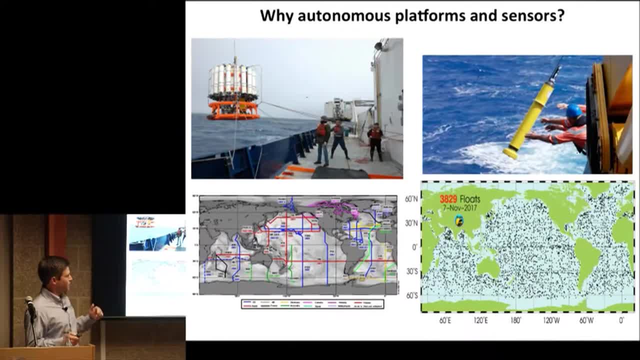 hope that you can do it, And so I'm going to talk a little bit about the Argo program in a minute. But why autonomous platforms and sensors? I mean, I said that the space scales are challenging and difficult, I mean the other. 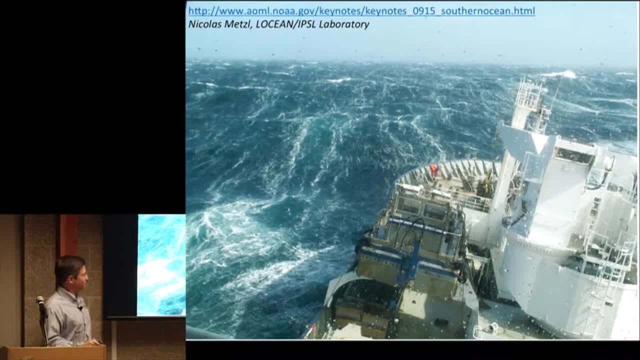 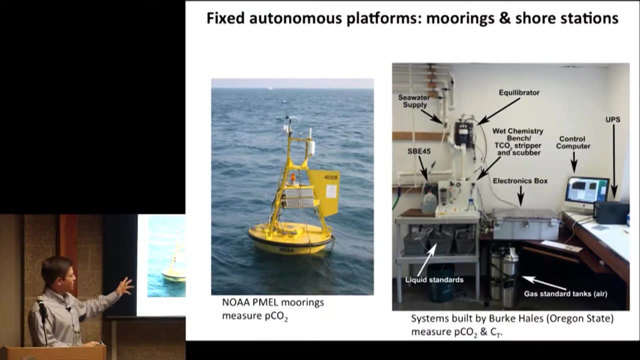 reason is just that It's extremely- and the Southern Ocean, for example, is really- difficult to work in, right? I don't want to be there. I'm just going to give you a few examples with photos of the types of platforms that are being. 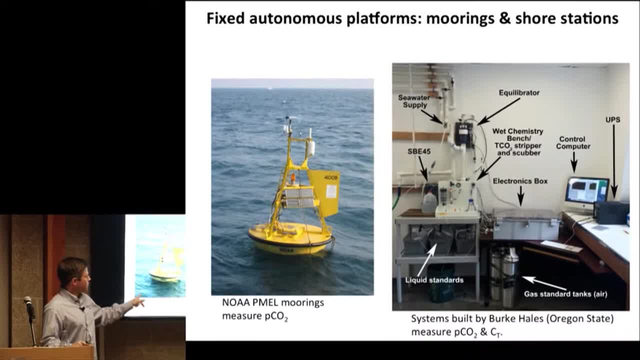 deployed autonomously. Moorings are currently the most widespread autonomous PCO2 measuring platform. if you're not counting underway vessels, There are- I don't know the exact number I'm going to say- approaching something like 50 moorings. 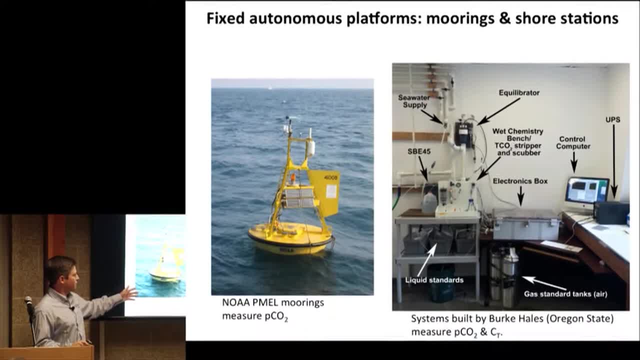 measuring PCO2.. Most of those are operated out of the Pacific Marine Environmental Lab in Seattle, a NOAA lab. I've been working with one of these systems lately. Burke Hales at Oregon State developed measures two of the CO2 parameters. 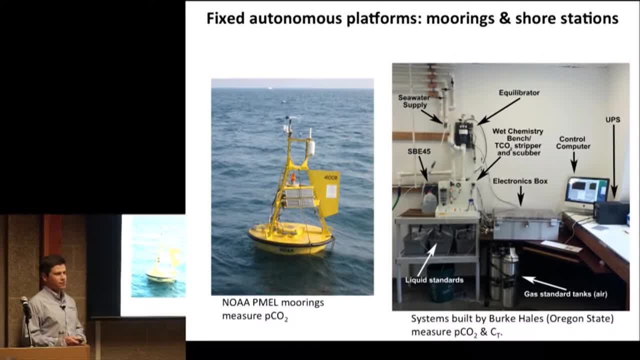 And these are located at a handful of aquaculture sites along the West Coast. There's one in Carlsbad that my group helps to operate, So this is a short. this is an underway shore station. It's continuously pulling water out of an aqua farm, providing 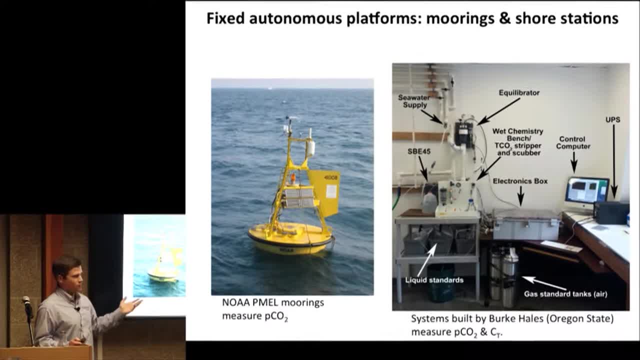 the chemistry measurements in real time, hopefully to the shellfish growers. They might be able to use that for something. Maybe they could make a decision about whether or not they want to shut off their intakes because there's this low CO2, high CO2. 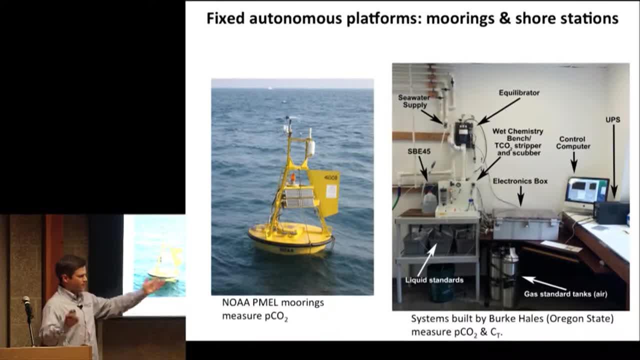 event- low pH event, Say there was an upwelling plume that came by and maybe they don't want to bring water in for a day because of that, And that's actually been shown in Oregon to be a factor. More exotic platforms that we're beginning to use to 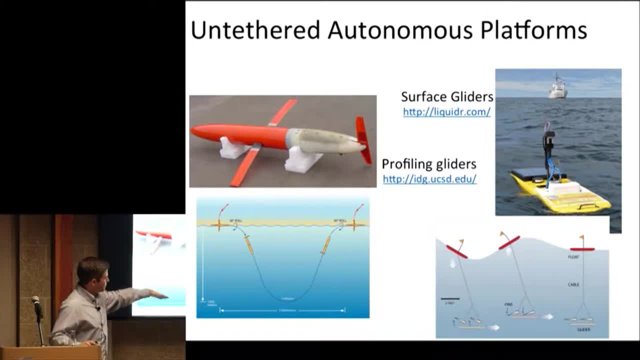 observe the ocean include things like gliders that can go down and come back up in a different place by controlling their buoyancy and their pitch, These surface gliders- so we have surf island gliders and surface gliders. They've made some recent progress. 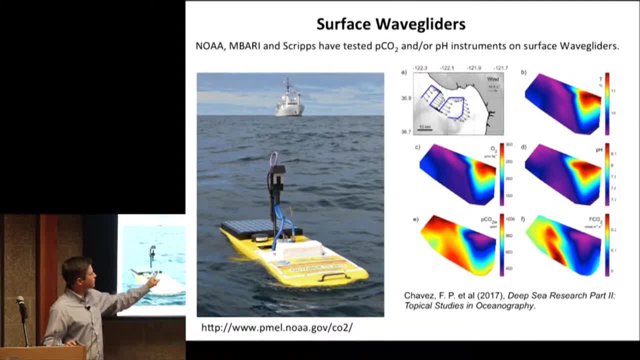 in putting pH and PCO2 sensors on surface gliders. We've worked in this area a little bit. The guys up at MBARI have probably done the best job and they have this really nice figure showing this little section of the northern Monterey Bay. 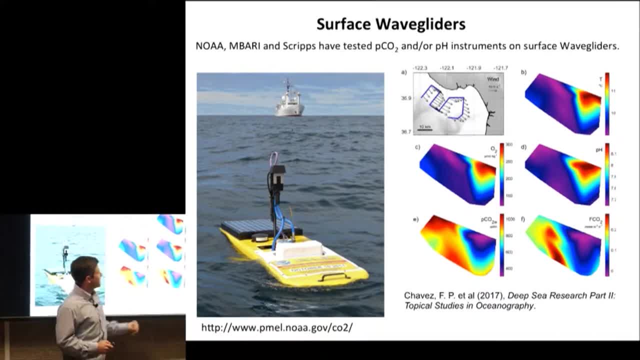 where they've got what appears to be a pretty intense phytoplankton bloom happening, which I think all happens regularly right in that area. So that's why you have this really high pH and a high oxygen and a low PCO2.. That's the hallmark of a phytoplankton. 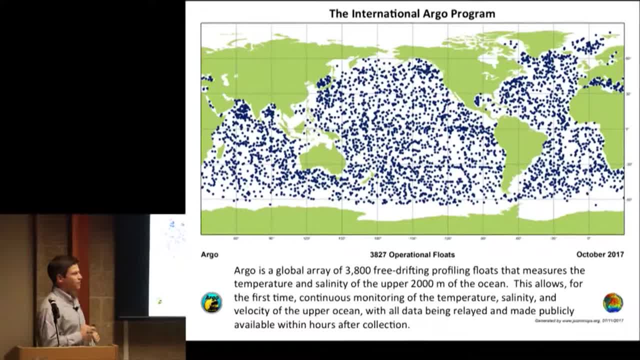 bloom. So I want to close on a few things about the Argo program. I think you've already heard about this. Margaret Linen showed at least one slide on this, but this is my opinion, the most successful global observing system that has ever been. 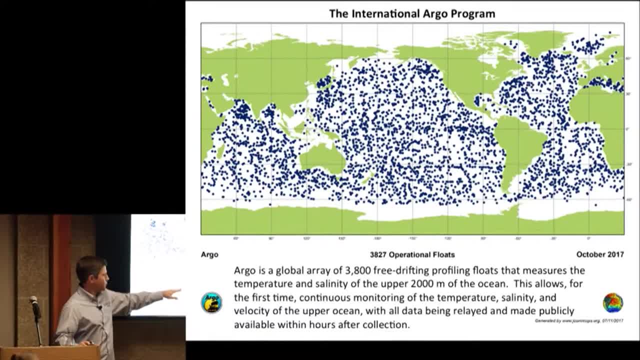 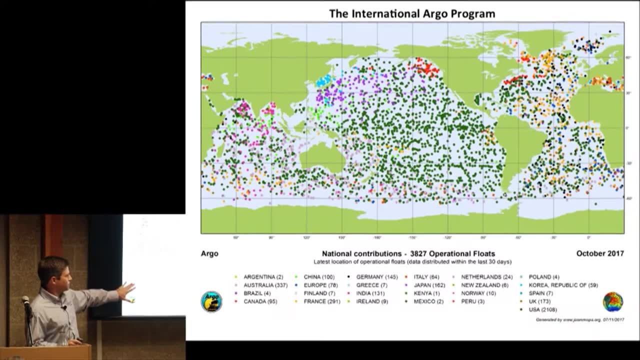 built Currently over 3,800 of these drifting floats. This is in the last 30 days. how many profiles have been done? This is a multinational program. I'm showing 25 countries here that are deploying these floats globally The way a profiling float 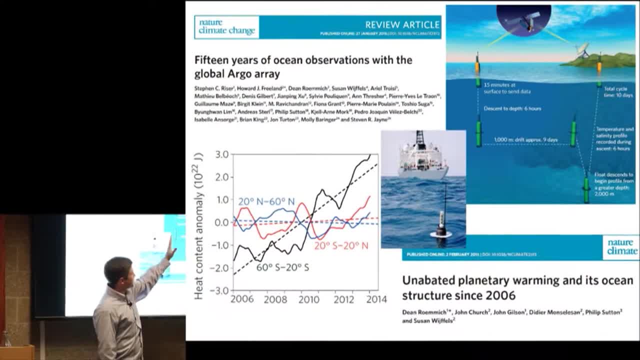 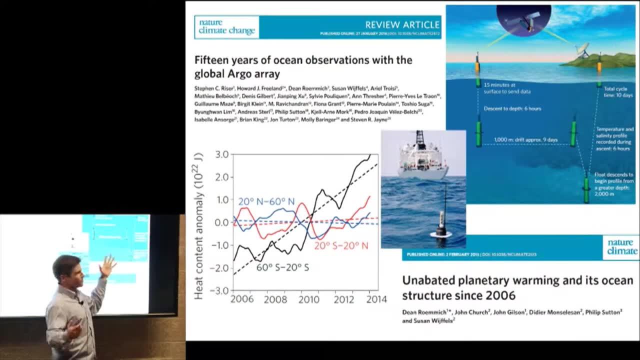 works is it goes down to one kilometer and it just drifts dead in the water for about nine days. Then it turns on and it drops to two kilometers. It turns on its sensors and it comes up to the surface measuring temperature, salinity and pressure. 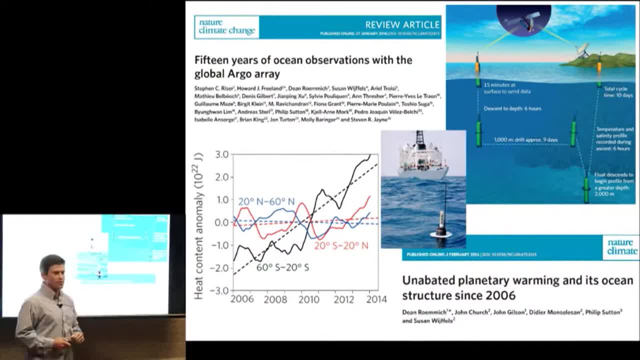 and at the surface. it sends its data to the satellites and we get it in real time. It's amazing. This is how we actually have been able to measure the global warming signal. We could not measure global warming until they built Argo, because over 90% of the heat due to 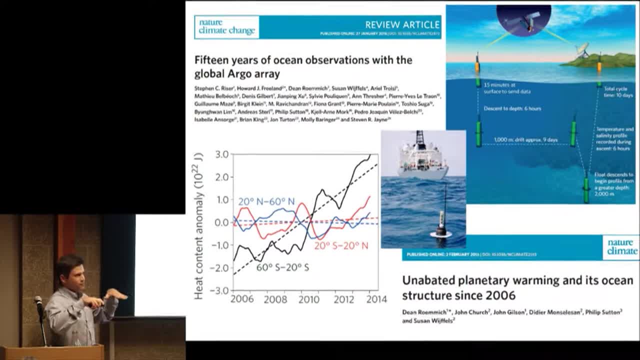 global warming is in the ocean, but it's not all in the surface ocean, It's in the upper thousand two thousand meters. So until they could build a global system that could profile that over years, they couldn't actually parse out this heat content of the total global ocean. 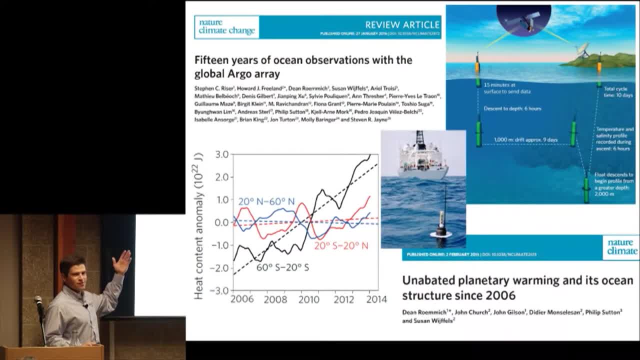 Atmospheric measurements are meaningless if you're trying to track the global warming signal. They're just the artifact of what the ocean is doing. They've been able to show that the southern ocean, the black line here, is actually taking up the bulk of the global warming signal. 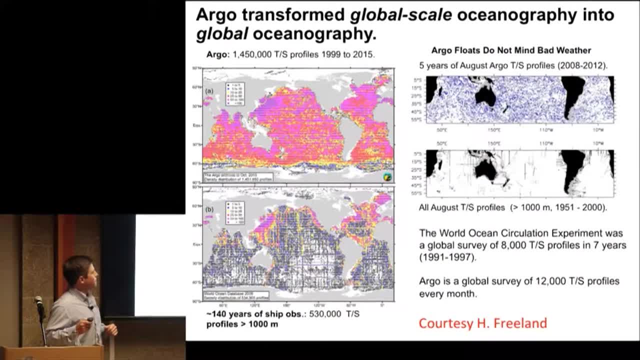 at least since 2006.. And just to kind of drive that point home and make: I love hydrography programs, so I don't want to say bad things about them, but it's really just amazing when you contrast the number of temperature and salinity measurements. 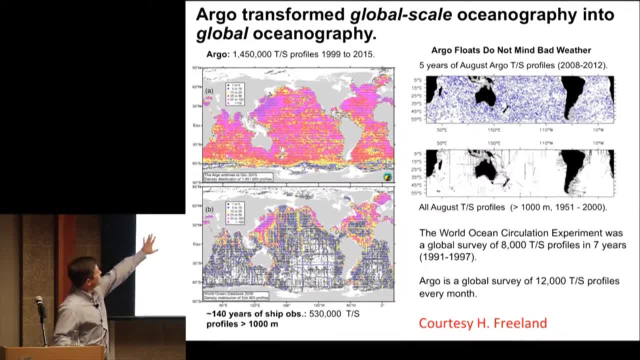 made in 140 years to what Argo does continuously. We're talking about orders of magnitude differences. So something like 8,000 measurements in one of these global observing programs Over 7 years versus 12,000 every month in Argo. 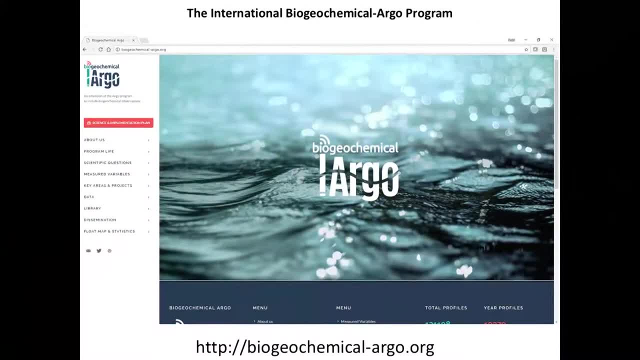 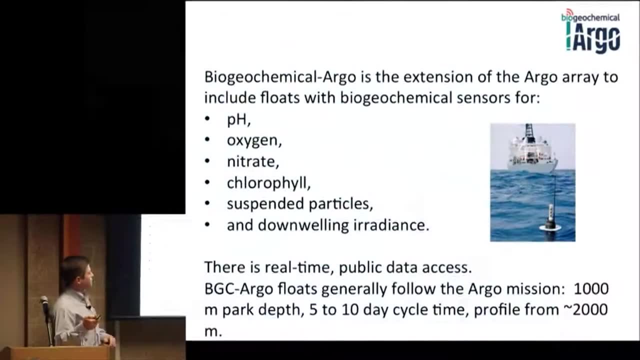 The reason I'm talking to you about Argo in an ocean acidification lecture is that we're now building bio-Argo, biogeochemical Argo. This is adding pH sensors in particular, which is what I'm involved in. I've also worked on. 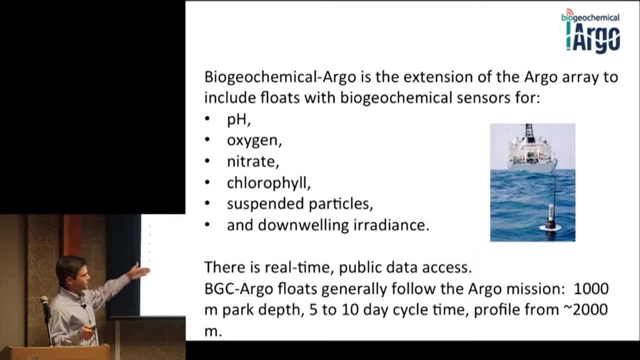 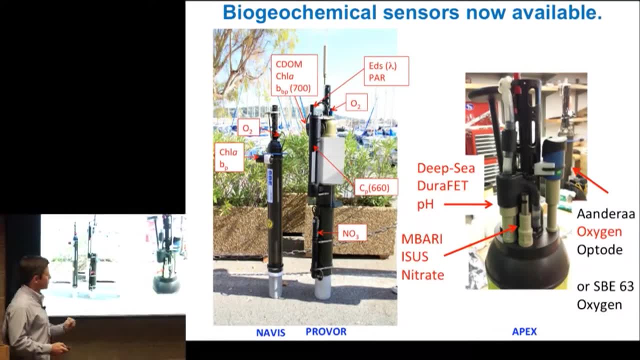 oxygen some, but a variety of other bio-optical sensors, including nitrate. Here's the durafet that I mentioned earlier on a profiling float. This is work that was led by Ken Johnson's group, my former post-doc advisor at MBARI. 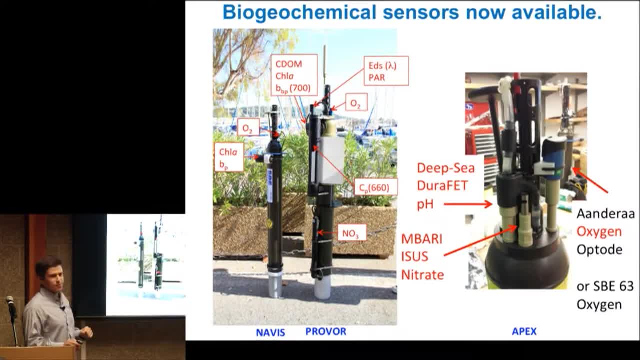 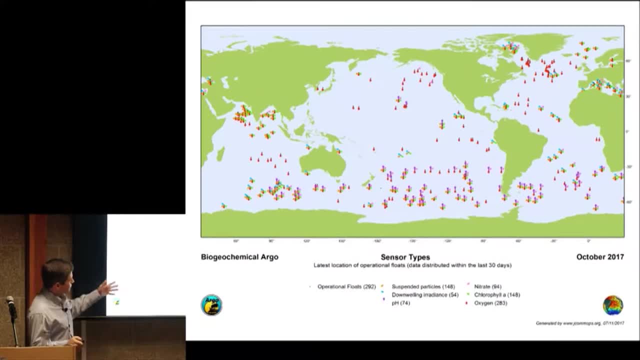 These things are just now decked out with six or seven different biogeochemical sensors and I think the next slide, if I can get it, shows currently. I downloaded this yesterday. it's showing all the bio-Argo floats in the array and what 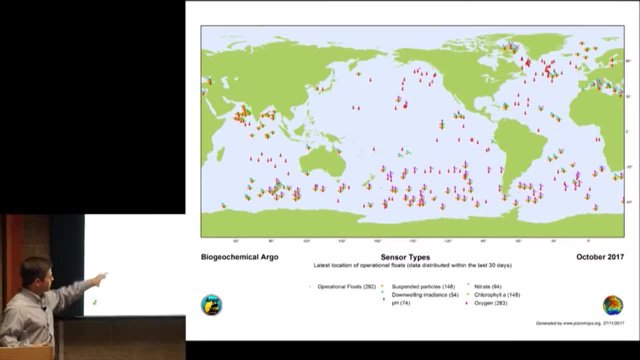 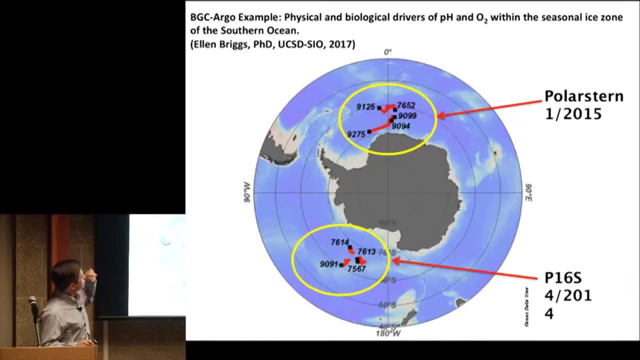 measurements they're making, but we've got about 74 pH measurements out in the southern. they're almost all in the southern ocean right now. This is through a program called. I don't know if I have it in here. it's in the next one, I think. 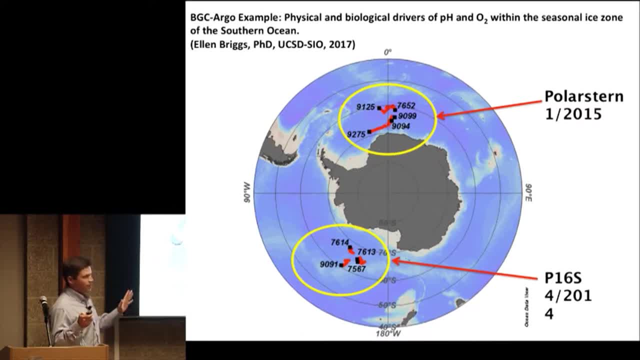 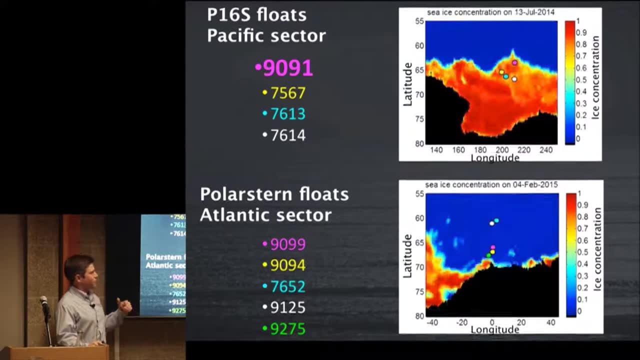 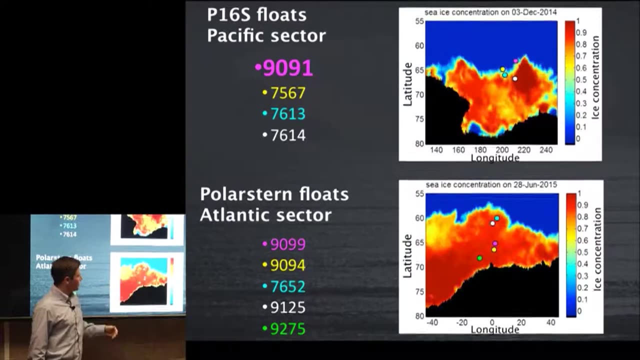 the SOCOM program. I just have a couple of examples. I'll try not to run over, but this is one of my graduate students working on profiling floats under ice. She wrote this paper where you can see the ice zone growing and these are the locations of floats. 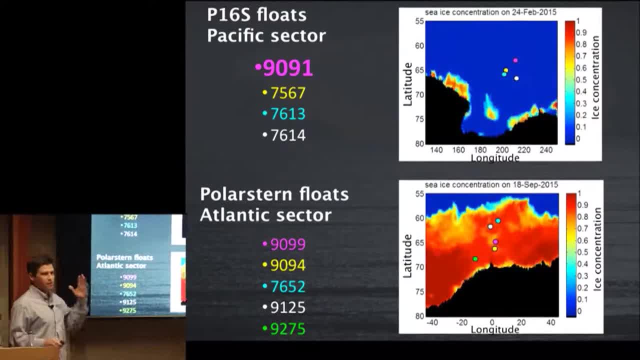 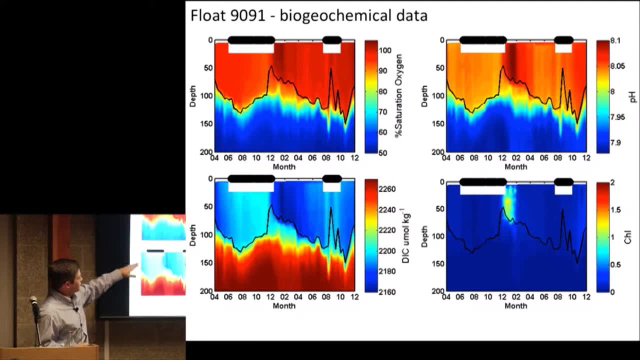 They go under the ice for the entire ice season and then they come back out and they send up their data. This is a year of, or it's actually one and a half years, so you've got two ice seasons of the oxygen and the pH and we've 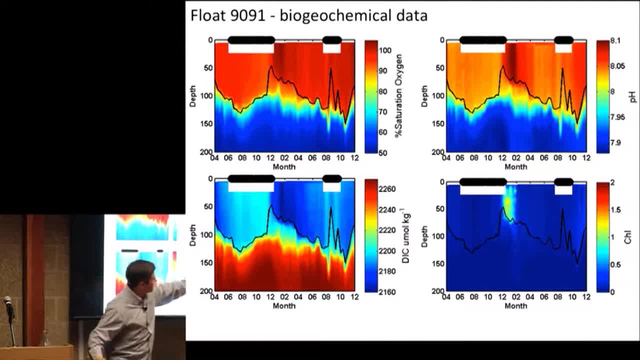 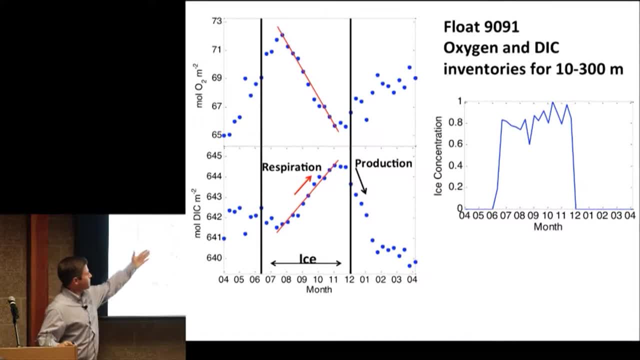 derived the dissolved inorganic carbon from the pH. in this example You can see a phytoplankton bloom happening right there. so this is the upper 200 meters. We can start to do things like assess rates of plant growth and respiration. so this is plant respiration. 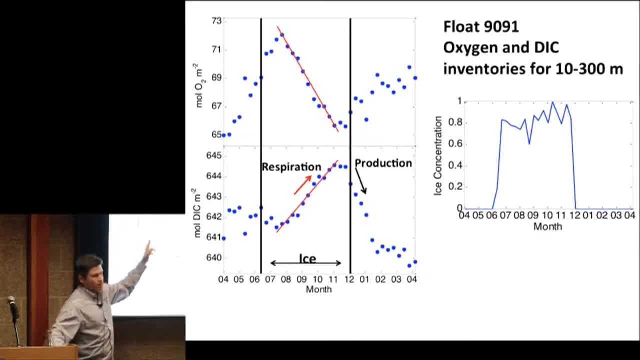 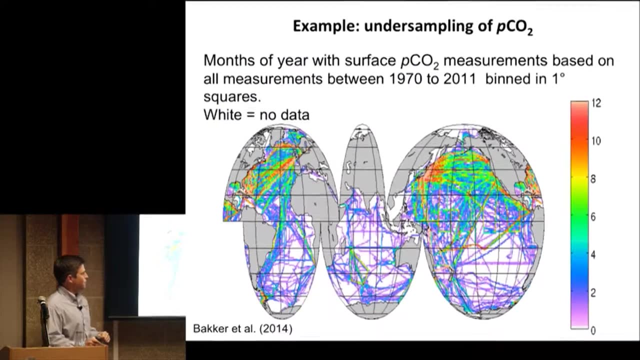 driving this line up, driving the oxygen down underneath the ice, and then the production drives the oxygen back up and it drives this dissolved inorganic carbon back down. So starting to use these biogeochemical floats to look at rates of production and respiration in the ocean. 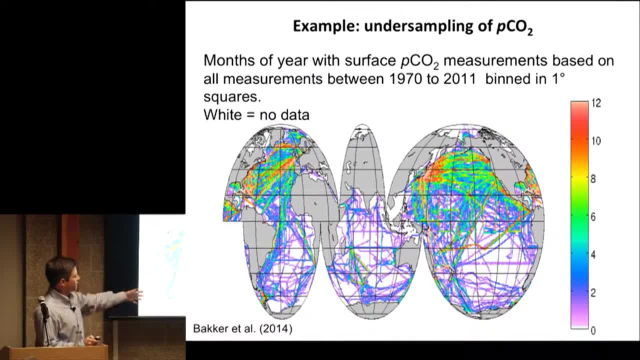 Another example that's coming out of BioArgo now. this is similar to the version that I showed you of all those, the PCO2 measurements, the 21 million PCO2 measurements in the ocean, except this now shows the number of measurements made along. 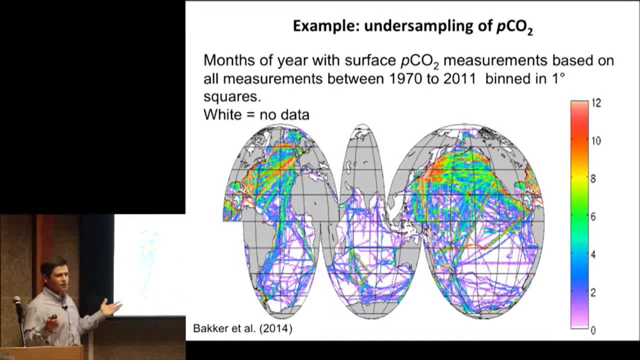 those lines, which is not so pretty. The other one showed the actual PCO2 number, but when you look at vast areas of the ocean that only have one measurement in a given month of the year or one month of data, one measurement in one month of the year. 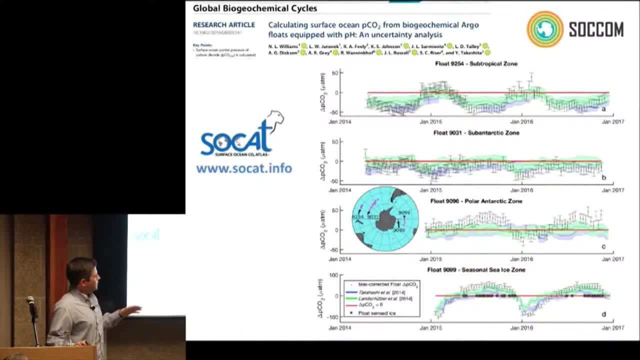 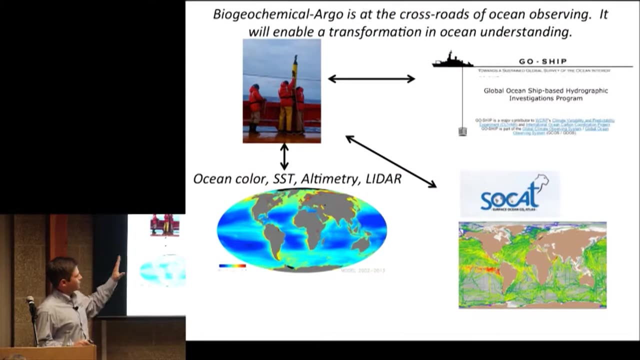 that makes it very hard to build climatologies, and they're now beginning to use the pH sensors on these floats to derive a PCO2 number that can compare with the climatology, and the short story here is that it doesn't always match, but they are working together. 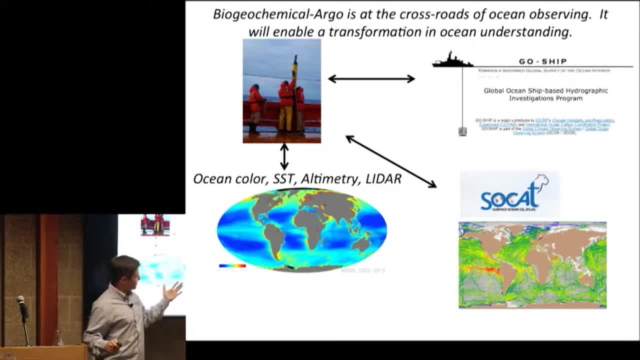 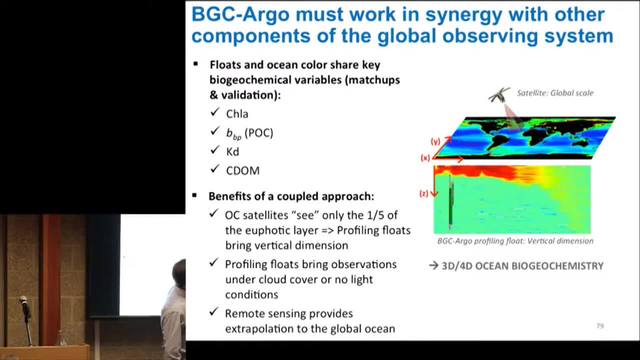 so it's not that the floats would replace the underway measurements. it's really that they would work alongside each other to improve each other, and you can think about this like this satellite picture that I showed. the idea is, you're bringing it into the Z dimension. we want to bring it. 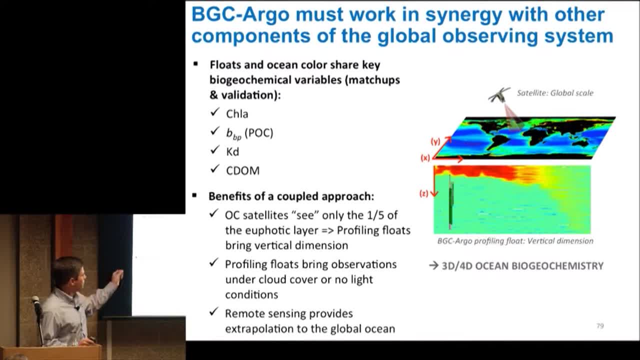 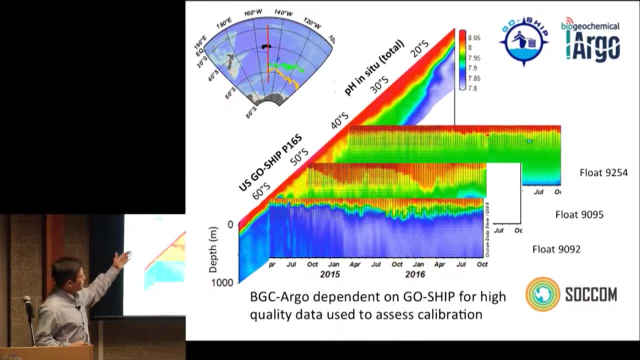 below the surface that the satellites are sampling. they're just looking at the upper, really the one-fifth of the euphotic zone. So GoShip, for example, the hydrographic programs are deploying these floats and, along their lines, making measurements that we can use to 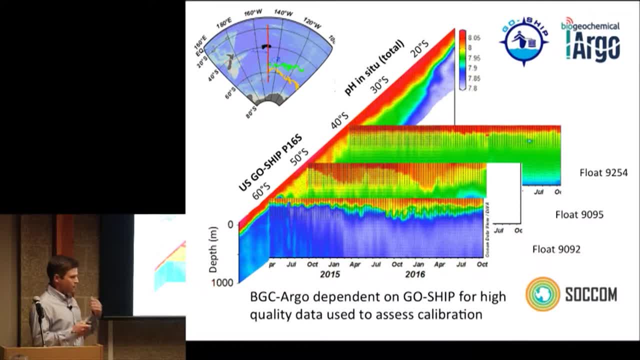 help calibrate and check offsets in the sensors. so you really only get one shot at that. once the sensor is deployed it's gone. so extremely important to be synergistic with these ship programs to get even one good pH measurement so you can help make a traceable. 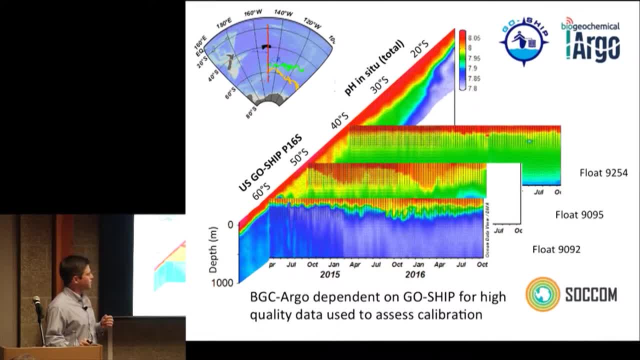 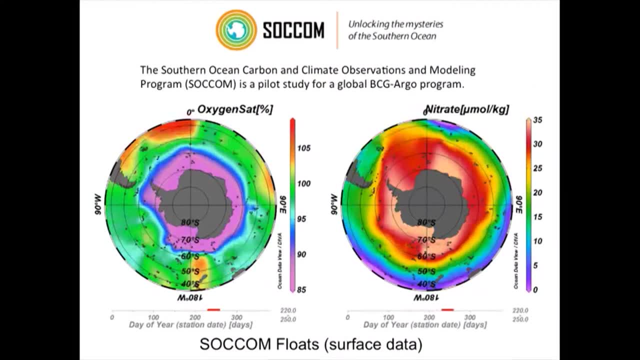 pH measurement that can be used in climate studies. And this is I'm pretty much done here, but I just want to show you kind of where people are at this is. I don't think this has been published yet, but this is some of the people working in this. 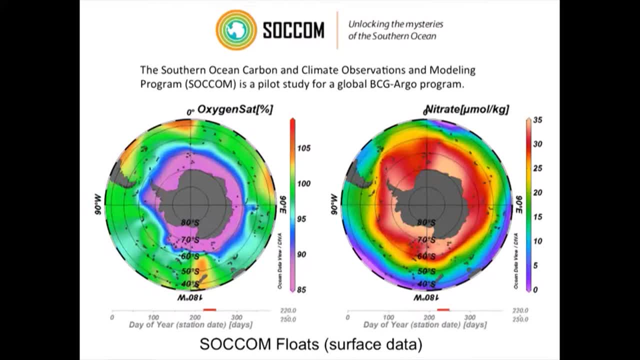 SOCOM program. so the Southern Ocean Climate Observations and Modeling program is the pilot study for the BioArgo program that I'm talking about. but these are the. this is the oxygen and nitrate sensor and these are just contoured values from all of the. 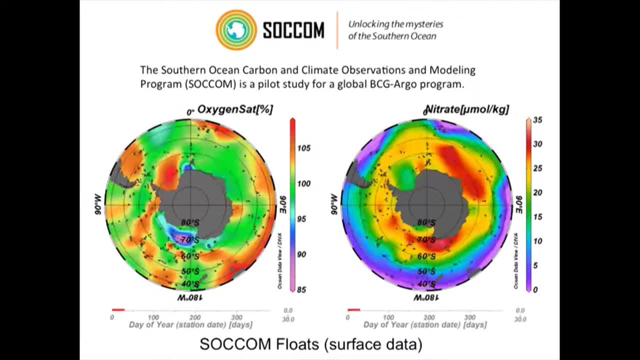 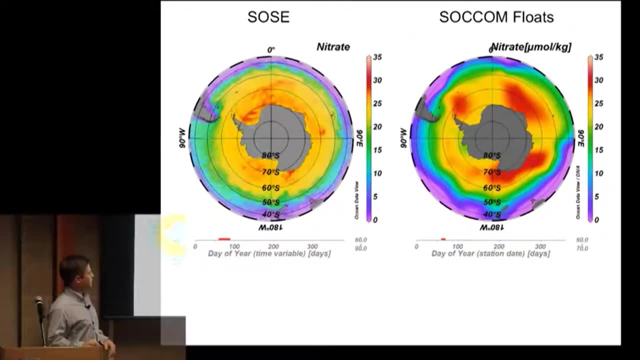 floats that are going around the Southern Ocean right now. and what do you do with this type of data? Well, you run an ocean circulation model- so people are running climate models- and you compare the model to the data and you use the data to